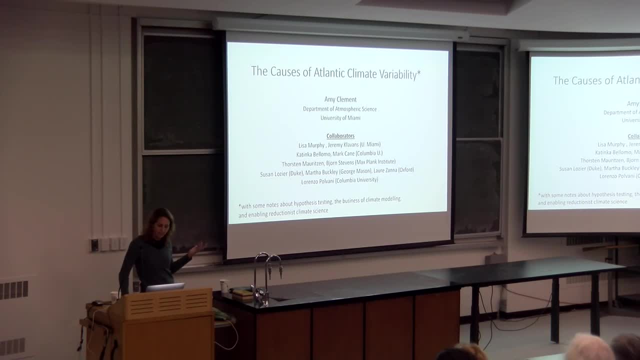 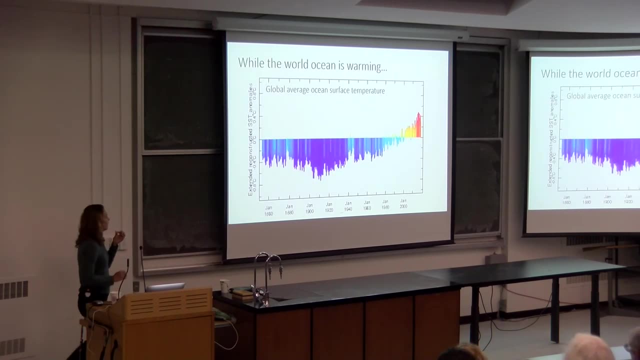 people in the physics community as well and give you things to think about, maybe even in your field. Thank you, your own field. Okay, so the world ocean is warming. It's not a surprise to anyone in, probably in this room. This is a picture of sea surface temperature going back to the 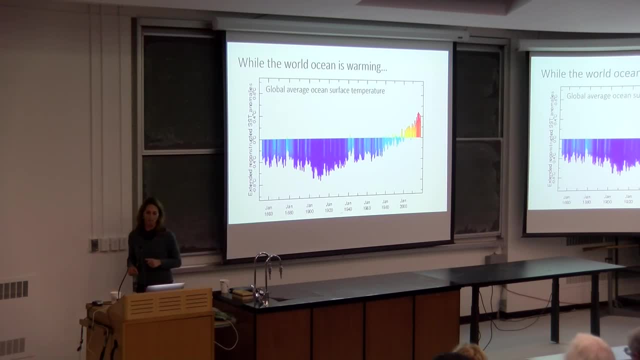 1850s, which is when we started a worldwide. we started a, the World Meteorological Organization, and the, the- basically the British Empire- started collecting observations from around the world oceans from volunteer observing ships, and that's how we know that the Earth is warmed. 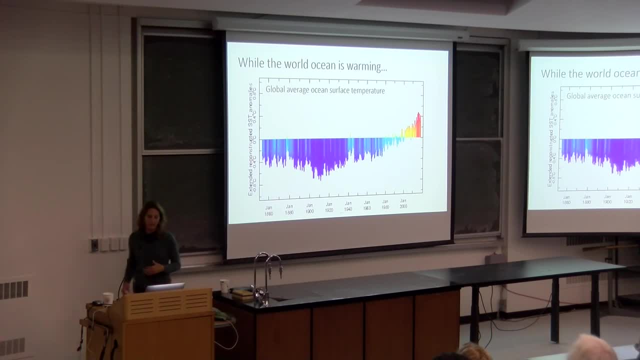 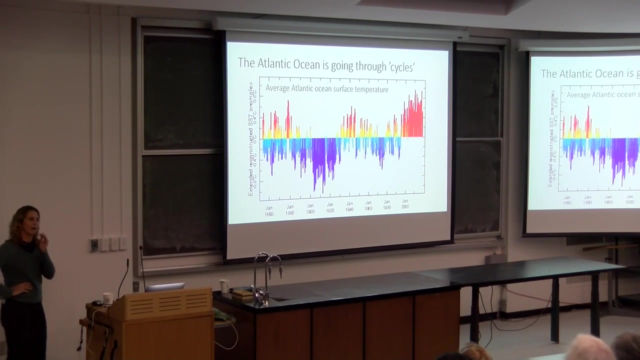 And you could see along history, with the present period being very anomalous compared to the entire observational record. So this is happening in the world ocean, but then in the Atlantic, which is a really well-sampled part of the ocean, there have been ships going back and forth across the basin over this entire time period. 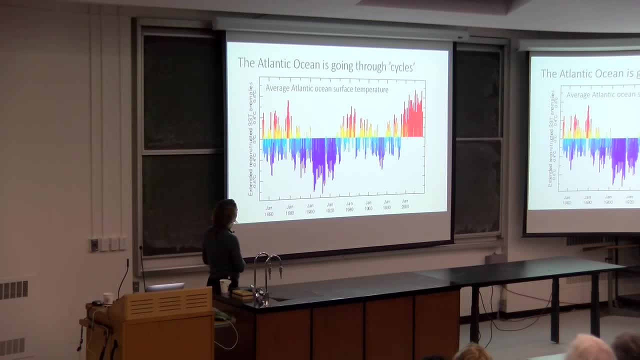 What you see, and this is just the average temperature of the North Atlantic, no filtering or anything. Each bar is a monthly value. The colors indicate just the magnitude. here, What you see, without any real data processing, are these cycles in the Atlantic. 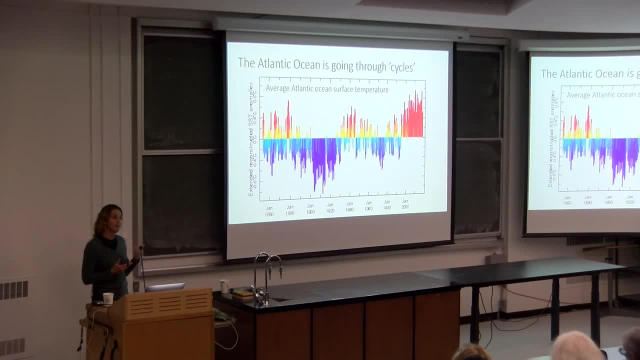 And they have approximate timescale. I will use the term multi-decadal, So by that I mean that for multiple decades the Atlantic will be in a cold state or a warm state, or vice versa. So these cycles, which now I'm showing again here, but, having detrended the data, 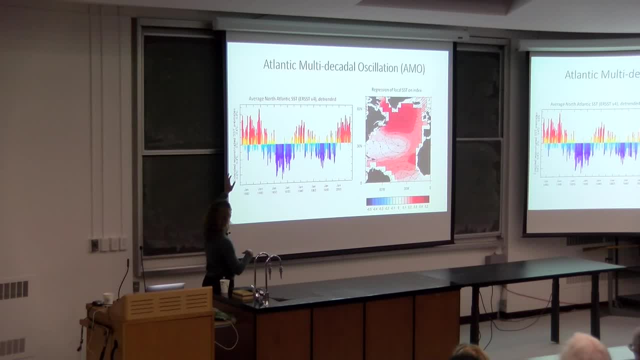 so taken out, this global warming trend- to emphasize the cycling of it- has come to be known- and I'll use this terminology here- as the Atlantic multi-decadal oscillation. It was actually coined by a science writer at Science who is not a scientist. 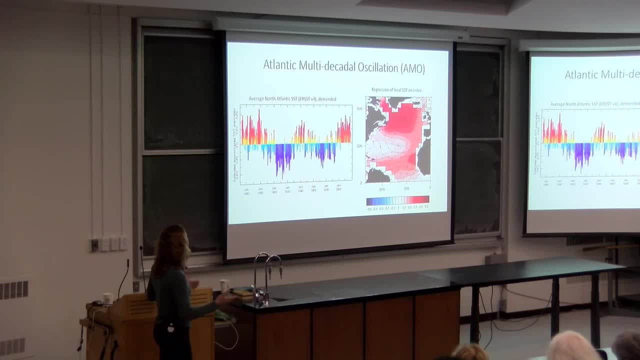 but was writing about the field and saying there appears to be this oscillation. It's a terrible term, I'm sure even worse in this setting, because as a physicist you're probably thinking: an oscillation has certain characteristics, But in this case, what the word oscillation is meant to indicate? that it varies. 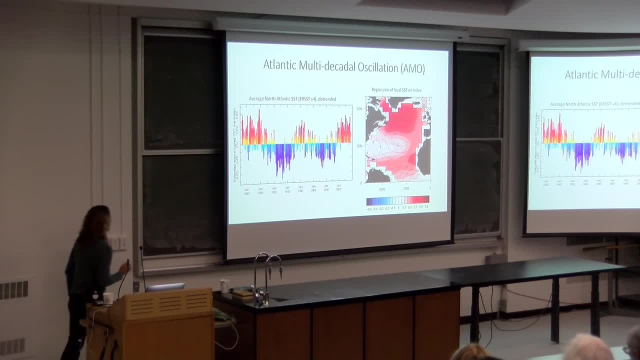 Nothing special. You might be tempted to look at this and say I think I see kind of a consistent period periodicity here And people tried to convince themselves of that. but let's face it, if it's a periodicity of like 60 years. 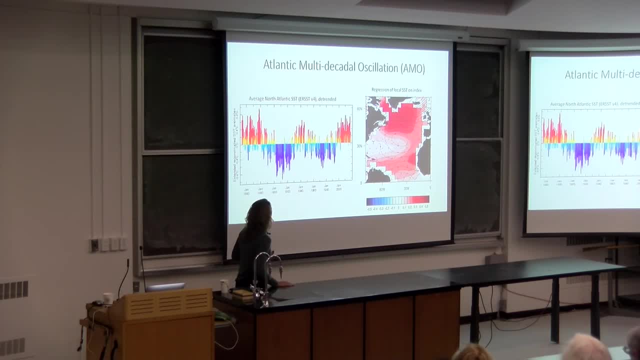 you have two realizations of it at best, And so it's, I would say it doesn't pass my statistical test of being a having a resonant period. This is a picture now a map, of the surface temperature pattern that goes with this index. 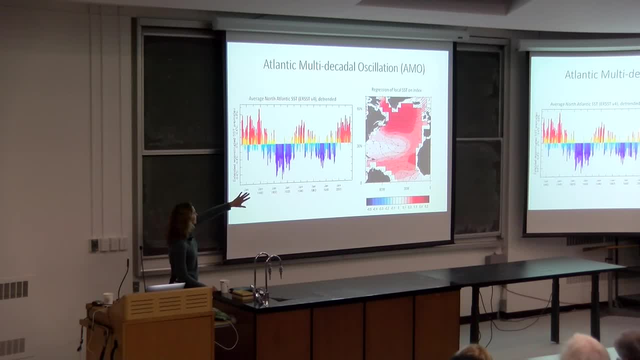 So if you take every point and regress the sea surface temperature at every point on this index, you'll get a pattern, a coefficients that look like this: Superimposed on this are changes in the winds. Those are plotted as wind anomalies. So, as you know, living here in Toronto, the prevailing winds are westerly. 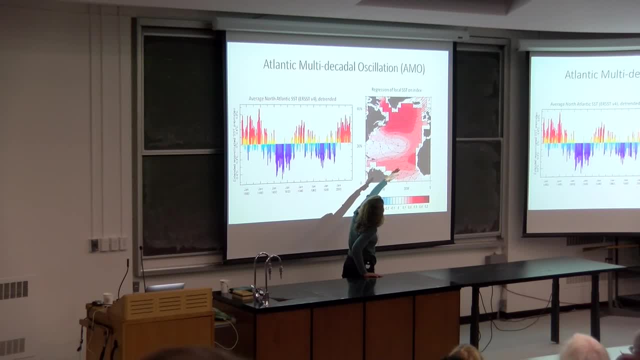 and that extends all the way out over the basin, Atlantic basin. So anomalous flow and this means weaker westerlies. And here I live down, here in the tropics, where the predominant flow is trade winds and so anomalous flow in this way will be weaker trade winds. 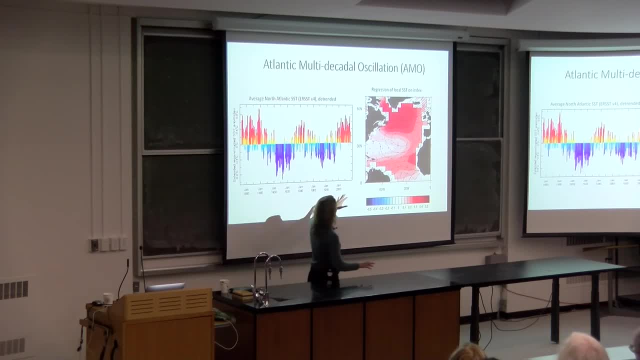 So this basically represents a weakening of the atmospheric surface circulation and you can also see in the contoured lines are the sea level pressure. So this shows that what is normally a low sea level flow but is very likely to be a weakening of the atmospheric surface circulation. 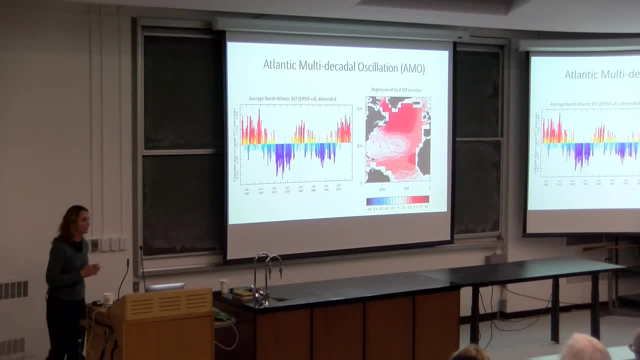 a big high pressure system sitting over the Atlantic which is making it dry and directing hurricanes around. it is weaker as well. So a coherent picture. We're going to come back to this same one, so you can kind of remember it, but it's really. 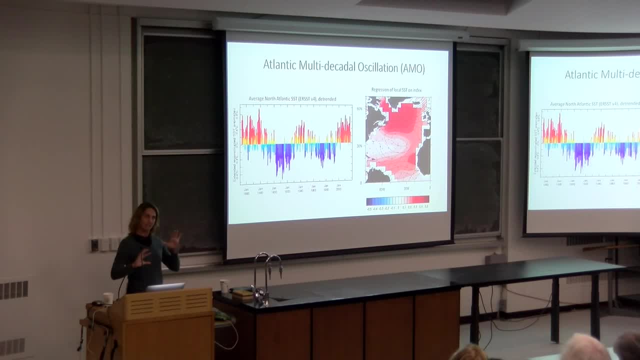 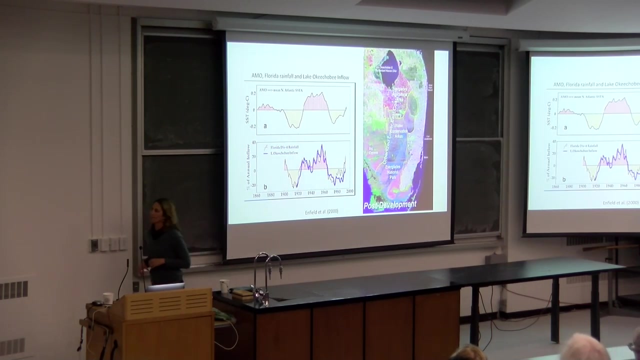 just to give you a sense of this, is the space and time characteristics of the Atlantic basin, with warming and cooling happening throughout. So why do we care? Well, this is a picture, just to orient you, from a Floridian's perspective. The left-hand panel is one of the first papers when this AMO terminology was coined in 2000.. 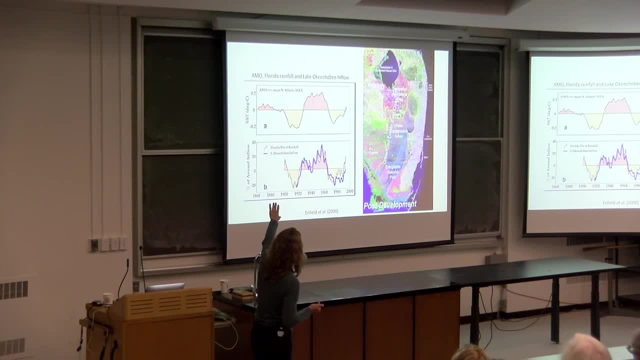 Looking at changes in rainfall in Florida. the top is that same index of the AMO, just based on North Atlantic sea surface temperature. The bottom is the temperature. It's the amount of rainfall happening in central Florida, which is actually what feeds into Lake Okeechobee, the largest inland lake in the United States, which is shown here. 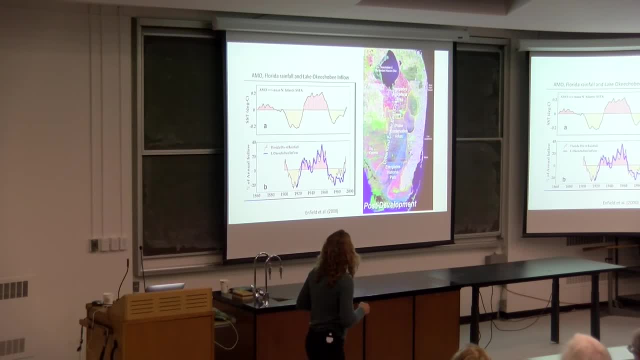 Now you might say: okay, well, big deal. From a Floridian's perspective- and I live right here- water and water management is life and death. In fact, I shouldn't say life and death, it's a little extreme, but it's existential. 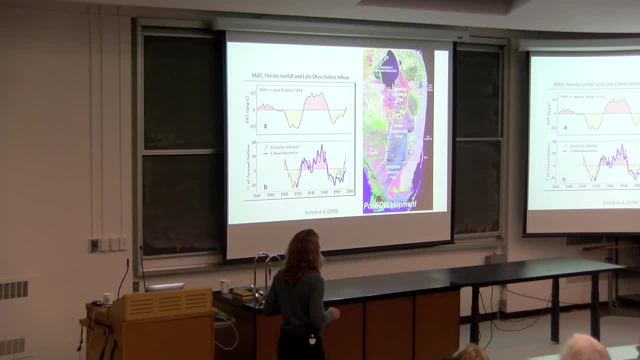 This is an all fully developed urban corridor of South Florida. 10 million people live here and they need water. This is the only. This is the Everglades, which is the only example of this ecosystem in the entire world. It was divvied up. It was. It was built up and canalized with Over the 20th century and then there was an act of US Congress to restore it to its natural state. There is a giant agricultural area which is: Did anyone hear about the red tides in Florida this year? 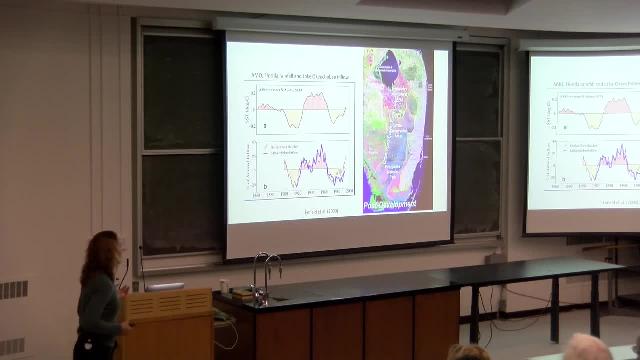 So blooms of cyanobacteria and living in the surface ocean, which if you breathe, they're really Really, Really uncomfortable And if you have any kind of respiratory issues it can be a real problem and it kills everything in the upper ocean. 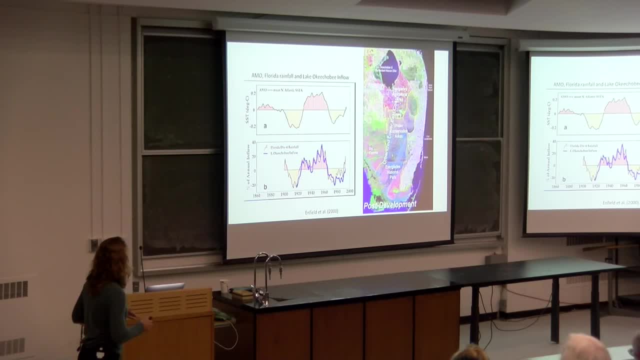 So fish floating up and It's really disastrous. And so the water managers in Florida are trying to manage the flow of water, serving all these different things and avoiding big pulses of water that bring nutrients from this farmland into the Biscayne, into Florida Bay, over here and into the Atlantic Ocean here. 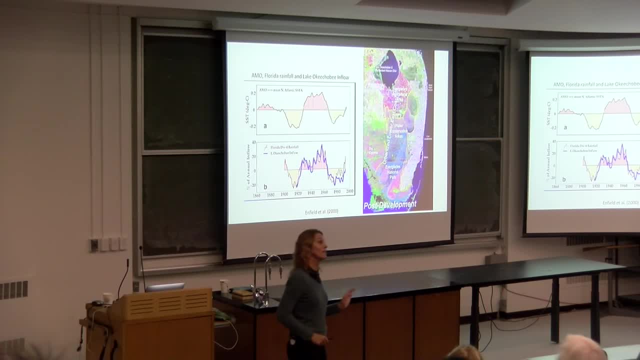 Really complex problem. Long tangent to say: we care about this because these kind of fluctuations of 20,, 30, 40% fluctuations of input into our water system make a really big difference in terms of life in South Florida for humans and non-humans. 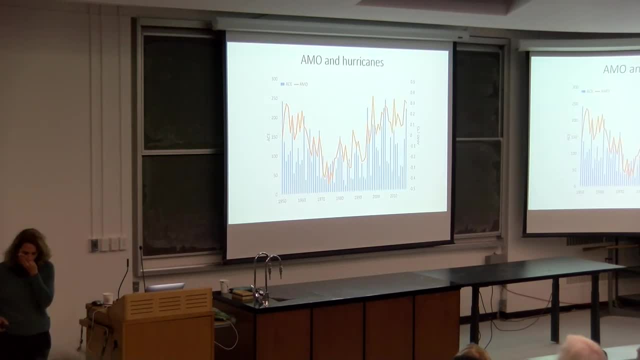 But maybe a bigger and even more charismatic problem is the changing status quo, Right Changing statistics of hurricanes over time. So again, this is the Now. in orange is the AMO index. So this is the North Atlantic Sea Surface Temperature-Based Index, here from 1950 to. 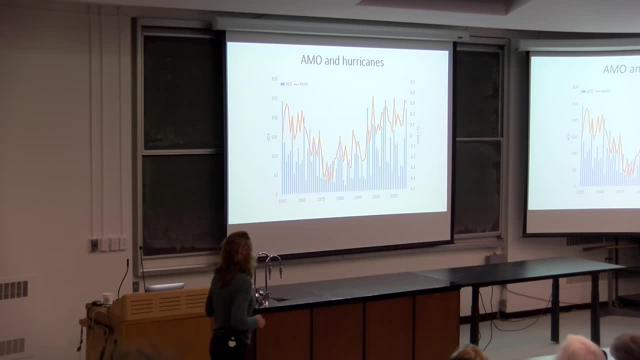 today, And what you see in blue bars are the total. It's a metric of the overall hurricane activity of the Atlantic Basin. This is a. So This, For example, this year in 2005, right here, was one of the most active years ever. 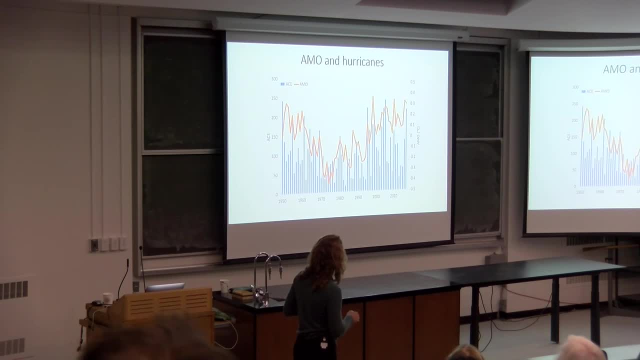 This is 2017, 2018 was also a very active year And you can see there's this cyclicity in hurricane, Overall hurricane statistic, Lots of intra-annual variability as well, but in overall changes that are really measurable, really observable. 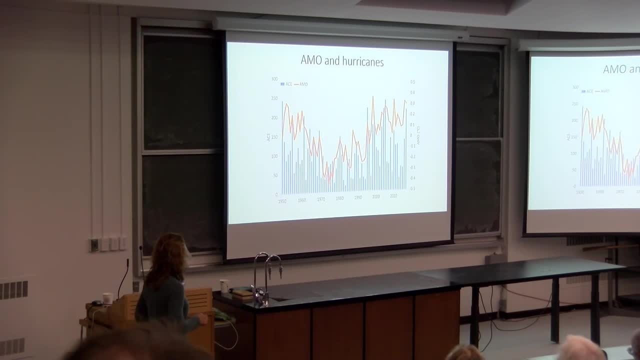 If you're used to this kind of hurricane regime, transitioning into this kind of hurricane regime really affects your way of life during the hurricane season in the continental, In the coastal and Gulf Coast US. Oh, I haven't done a very good job of convincing Canadians why you should care about the AMO. 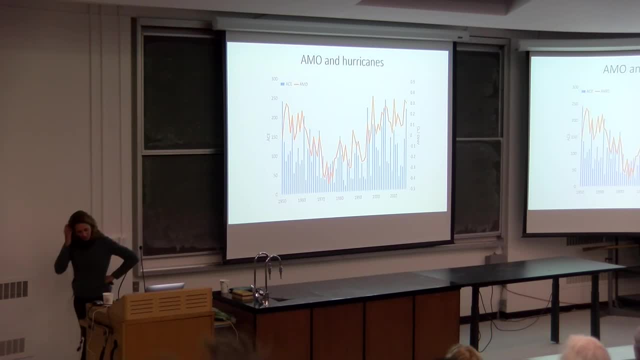 But there are impacts, I think, in the Arctic, which are, I think, in the Arctic? Yeah, Yeah, Yeah, Yeah, Yeah, I think there are impacts. There are impacts that are written about in the literature and there are certainly impacts. 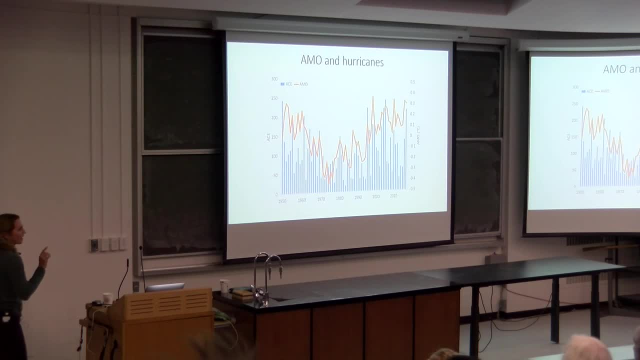 in European climate in the summertime There's impacts for those of you who are interested in North African rainfall. I'm still not quite getting to Canada, but Oh, okay, There we go. There's your hook, It counts. 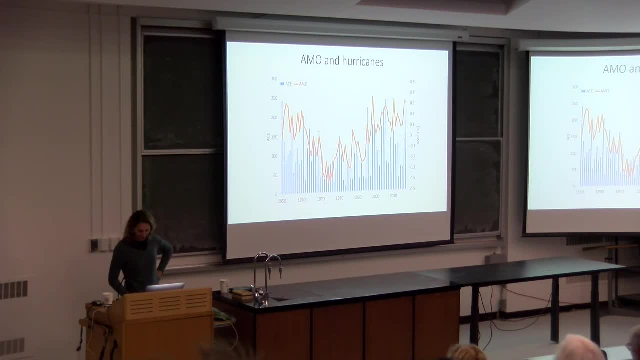 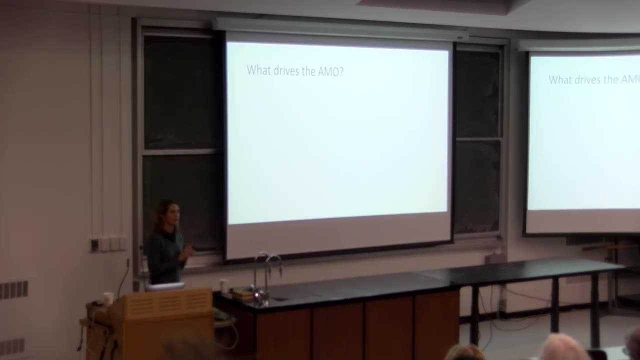 Okay. So we'd like to know, We all in, We'd like to know- what drives the AMO, What, What, What. What introduces this cyclicity that really is unique in the whole world ocean of this kind of multi-decadal changes that have big impacts around the basin? 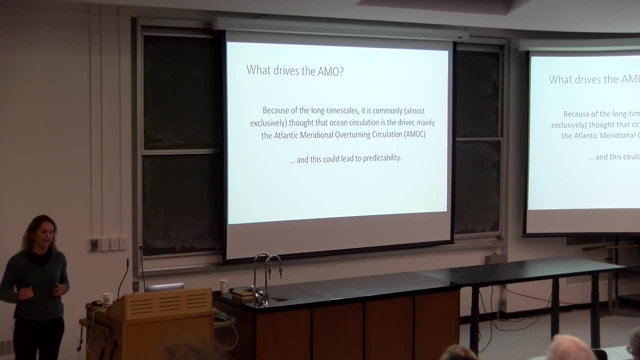 So I'll just say in words what is a summary of, I would say, decades of literature on this topic, which is that, because of this long time scale, it's commonly, or almost exclusively, thought that the ocean circulation is the driver And mainly the aspect of the ocean circulation, which is the overturning part. 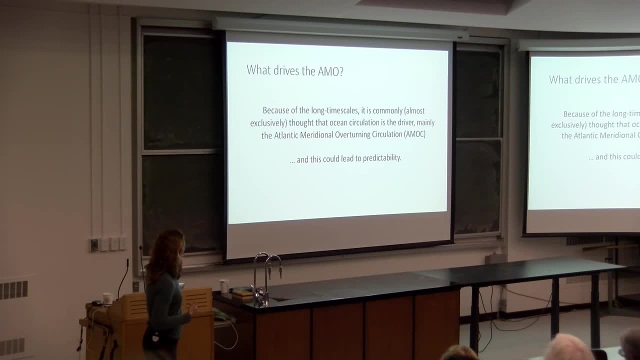 I'm gonna get into details about what I mean by that next, but we'll call- I'm introducing another acronym here- AMOC- Atlantic Meridional Overturning Circulation, And the idea here, and I would say the hope, is that, if you have 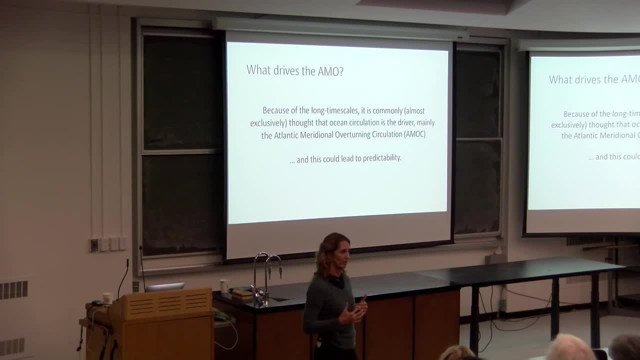 If the memory of the system exists within the ocean and it's slowly varying- that you can By By knowing the initial ocean state, you can have some predictability out to, let's say, five to 10 years. So insurance companies are really interested in knowing what the statistics of hurricanes 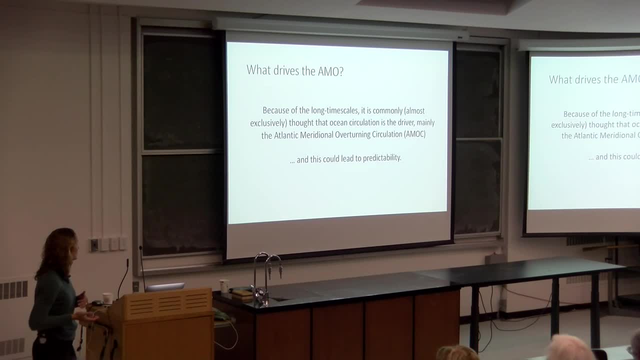 will be in the coming five years. It makes a difference And so it's kind of, I would say, the holy. One of the holy grails in the field of climate variability is to try to find, To mine those sources of potential predictability and think of it just like a weather prediction. 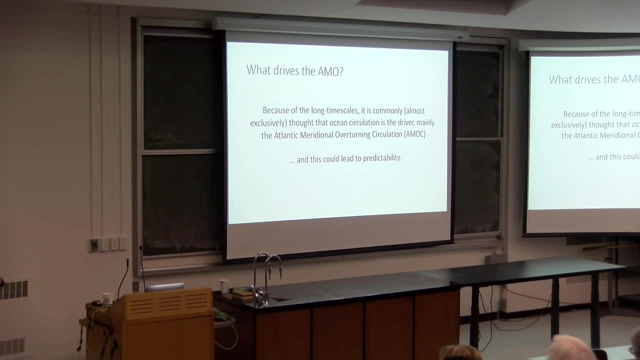 problem And the atmosphere. we know that the We can predict the. Knowing the initial state of the atmosphere, we have some predictability out about a week And then that predictability goes away because of the characteristics of the atmosphere In the ocean. the idea is knowing that ocean state we'll have. 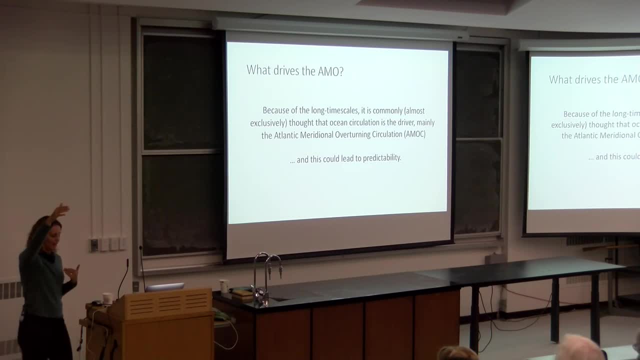 The ocean inherent timescales are longer and that we'll have some predictability going out years to Even Even a decade. All right, So Do I. We started at 4.10, right? Okay, Am I supposed to finish by 5?? 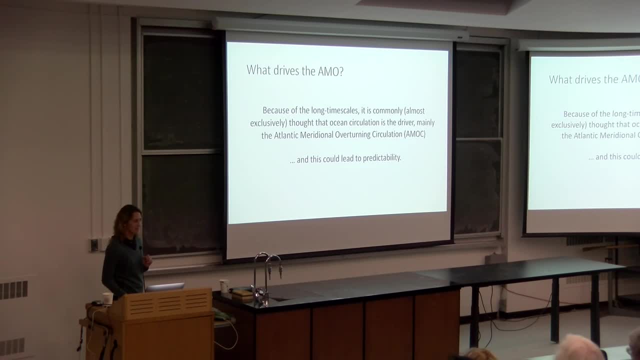 Yes, Okay. Silence means yes, Okay. All right, Then I'm gonna. I may not make it through the whole talk, but I'll get as far as I can. So AMOC: the Atlantic Meridional Overturning Circulation. 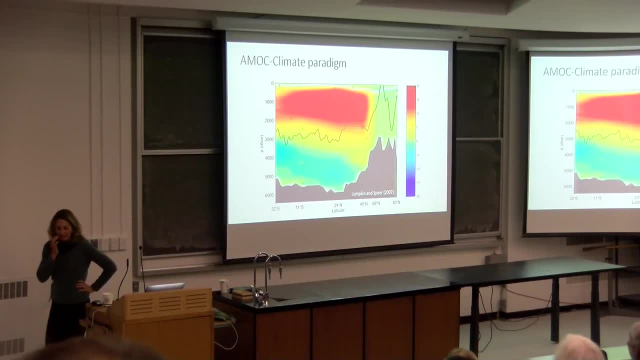 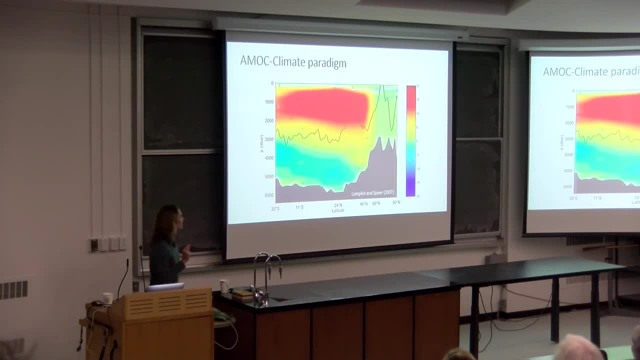 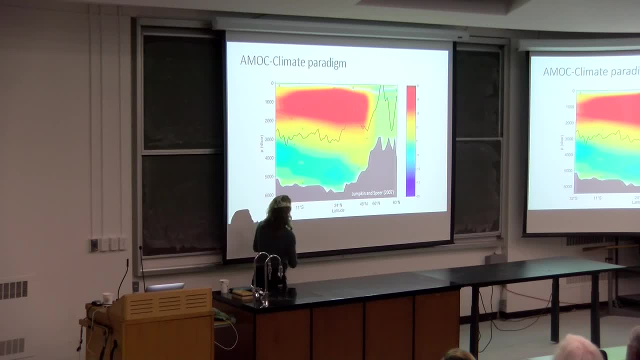 It's a stream flow. It's a stream flow. It's a stream flow. So positive values mean circulation like this. This is the depth latitude plane. Here's the equator. What you see is that, if you take all of the available observations of the Atlantic Ocean, 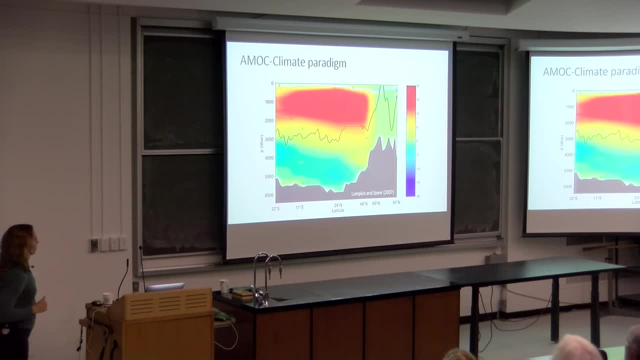 Circulation. you see that there's an overturning. There's water flowing to the north In an average sense across the basin. there's water flowing to the north, sinking in the high latitude and flowing out at depth out of the basin. 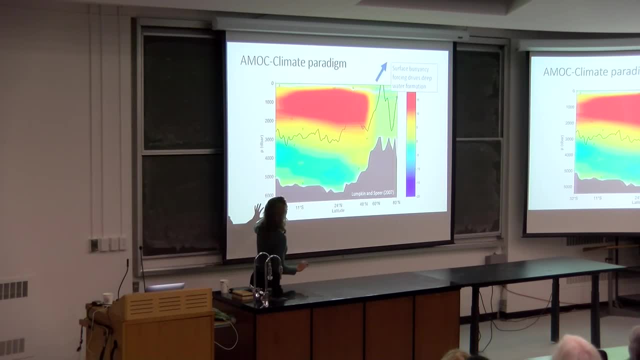 So the idea here is that this is a buoyancy-driven circulation, that buoyancy loss from a very warm ocean being under a cold atmosphere in the high latitudes means that this destabilizes the ocean column and you have deep water being formed or convection mixing surface waters, recently ventilated waters down into the deep ocean. Some of the first measurements, I think, of this were measuring oxygen levels in the deep ocean, which are really high in the North Atlantic because of this recently ventilated or any other ocean. So that's why the and this overall circulation is bringing heat from lower latitudes into the North Atlantic. 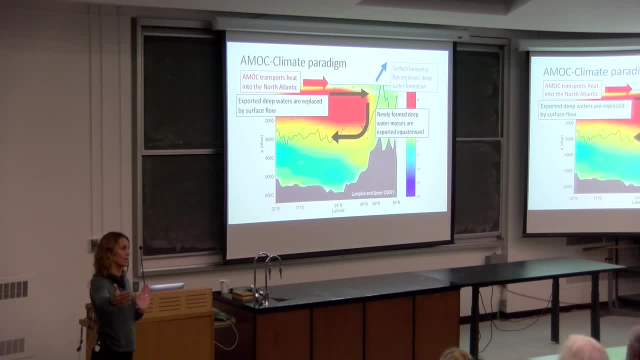 even across the equator. It's converging heat in the whole entire North Atlantic basin. so if you were paying attention and you saw the movies that I started this talk with, you should be saying: why is she drawing arrows that look so simplistic for the ocean when it's really messy out? 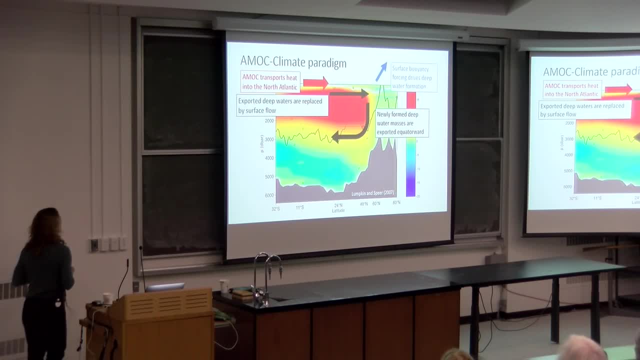 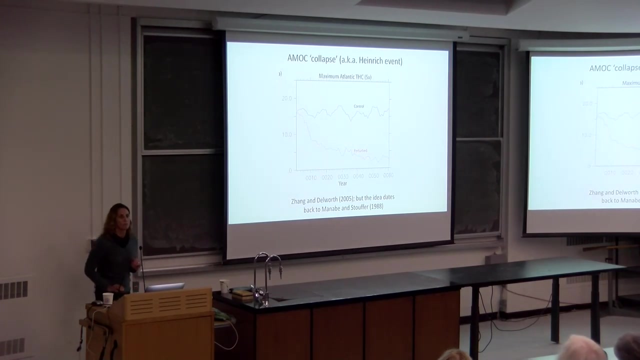 there and I am going there, but I'm telling you that this is the kind of cartoon textbook picture of how we look. we as climate scientists, many of us- have looked at the ocean, and I'm trying to argue that maybe we should be rethinking this. okay, so now, why should that matter for what I'm talking about? for these: 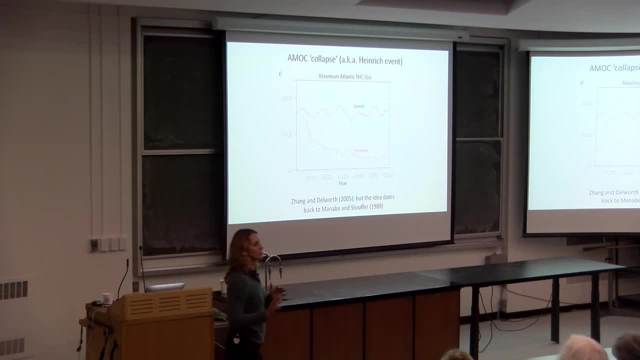 Atlantic multi-decadal cycles. so just very stated. very simply imagine that the circulation speeds up, it's going to bring more heat into the North Atlantic. if it slows down, it will bring less than the North Atlantic will cool. so the idea is that if you have variations, multi-decadal variations, in the 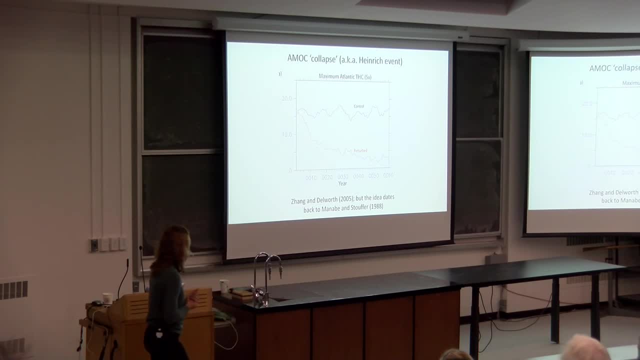 overturning circulation, that it will drive changes in the North Atlantic. so this is not a crazy idea. a collection of work that actually Dick Peltier was involved in over the years, I would say starting in the kind of late 80s, 90s, last century- that the ideas were formulated, being formed around the, the 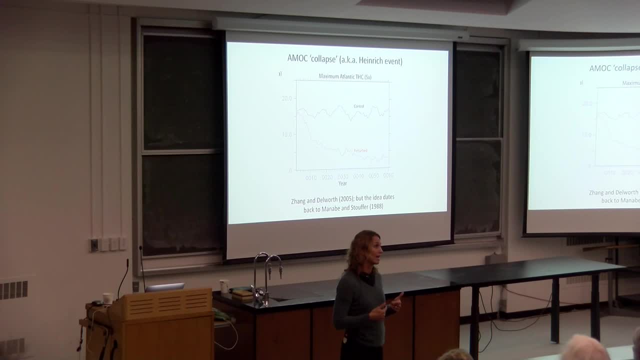 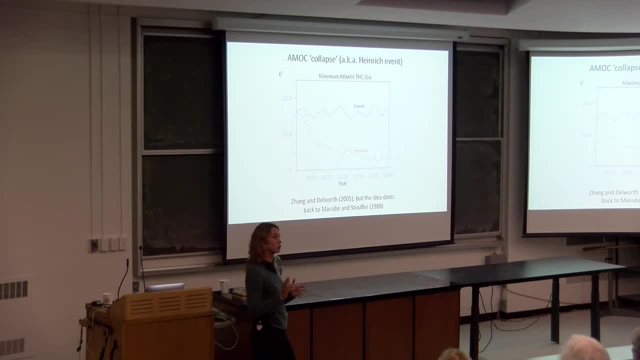 so there's evidence in the Paleo climate record for what are called Heinrich events. so they're extreme cold periods in the North Atlantic Ocean and if from observations I won't get into the details, but just if you want the details, you can ask Professor Pelletier. 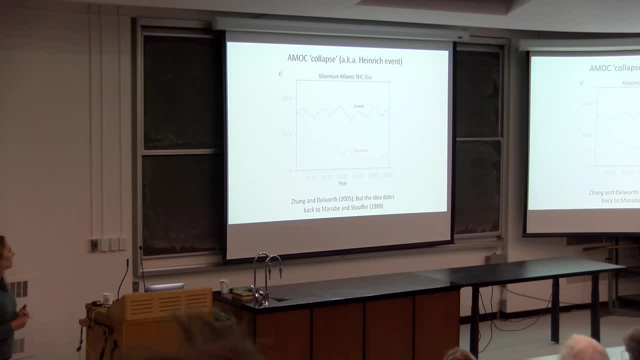 about it, Reconstructing the ocean circulation from proxies, from ocean sediments, that you can see that there was a really different ocean circulation at times when it was really cold in the North Atlantic. So it all kind of fits together. It fits together. 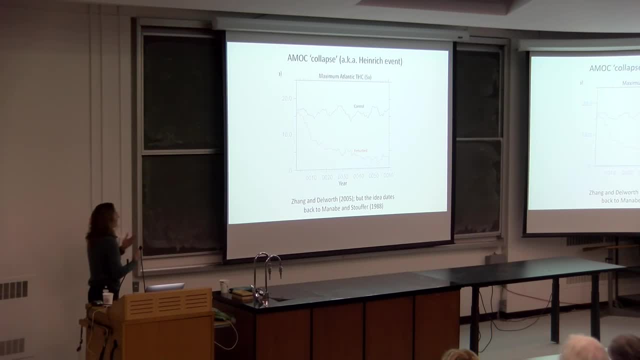 both mechanistically and from an observational point of view. Now, this is an experiment that was done with a model, a climate model. I realize I'm talking about climate models without having to introduce what they are, but that's coming. I just want to introduce the. 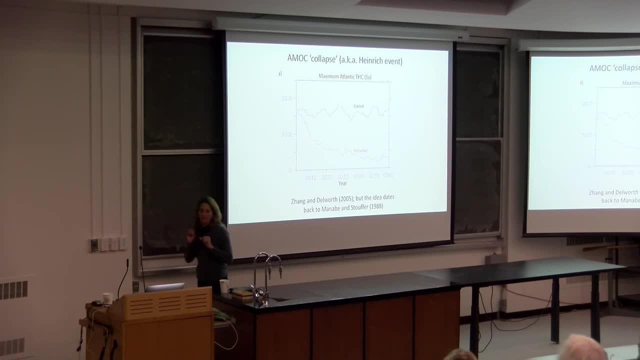 concepts here. If you take a climate model and you take ice and you melt it and you spread it over the North Atlantic Ocean, which is what we think happened during these Heinrich events- this AMOC will shut off, And that happens in climate. 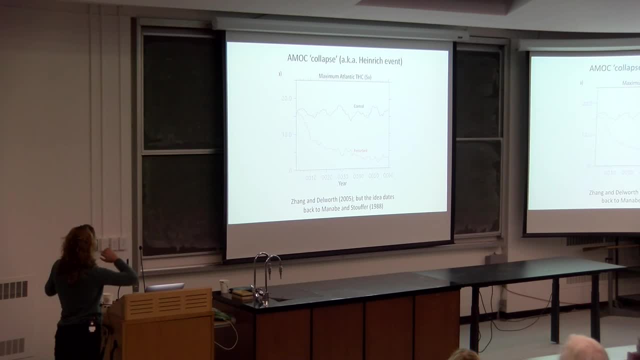 models. So this is a metric. The unit is spur drops and it shows that your climate model going along having some variability there. If you flood the North Atlantic with fresh water, which is done in this red experiment, it shuts down to almost zero overturning. 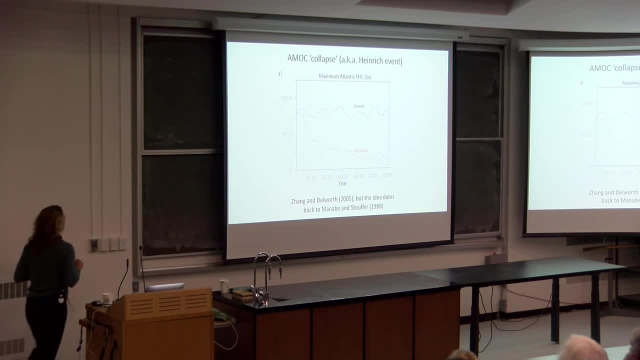 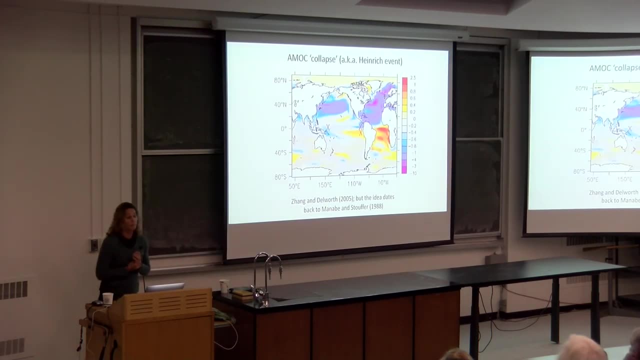 And these ideas go back to the late 80s with some of the first climate model experimentation by Suki Manabe and Ron Stauffer. This is the surface temperature that comes with a shutdown of this overturning circulation, and it looks kind of like. 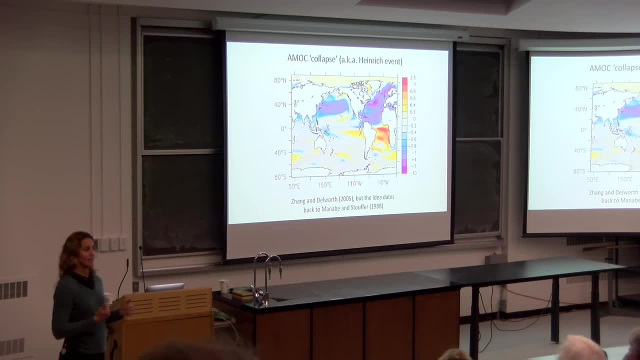 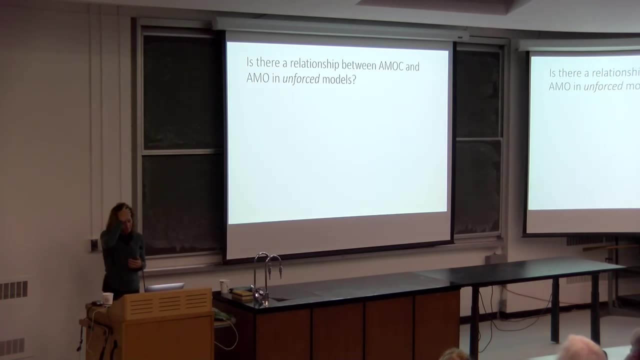 what I showed you for the observations, except the opposite sign: Weaker circulation, colder North Atlantic. Okay, everything's making sense. So now let's look at: is there evidence for a relationship between the AMOC and the North Atlantic SSD or the AMO in? 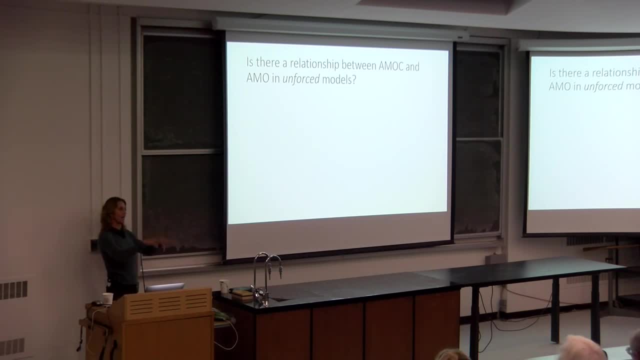 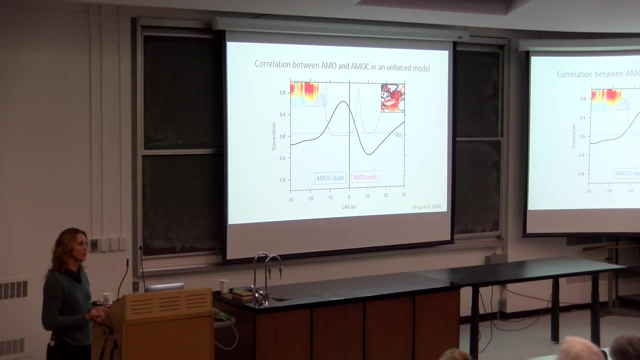 models when they're not forced with a giant pulse of fresh water coming out of the northern ice sheets. So this is where we start to get into. how do we use, how do we diagnose in our field what's going on? And a lot of ways we do is by looking at correlations between variables. 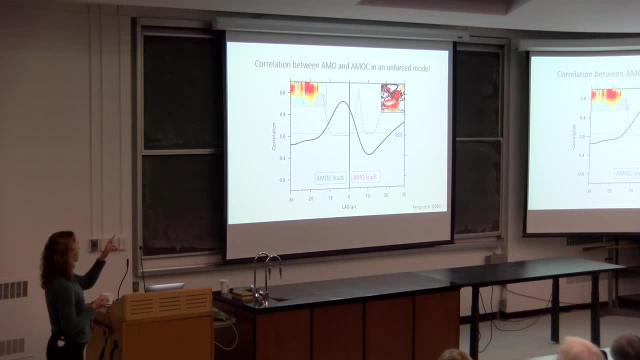 And what's shown here is a correlation coefficient between the AMO and the AMOC, which is which is with, as a function of lag. So it's a cross correlation function And the idea here is: okay, well, you can show that there's a relationship between them. That's nice. Then you can't. 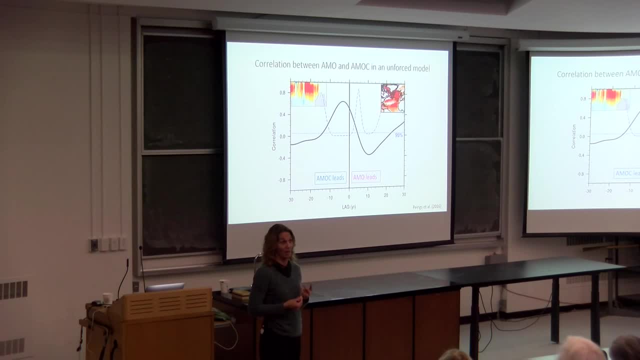 reject your hypothesis that they might be related. they are related, but you don't know what the causality is. Remember, correlation does not equal causation. But if you look at some lead lag sense that you may have some some idea that if one leads the other, that 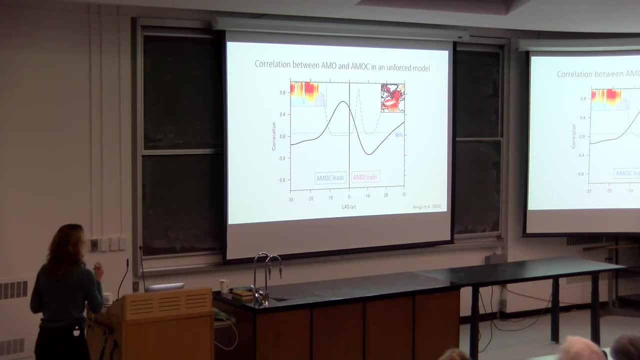 it has some information about causality in it, And so that's what's shown here When you look at a cross correlation function from some work earlier work that when the AMOC leads the AMO by a couple years. so the idea here is that you will a strengthening of 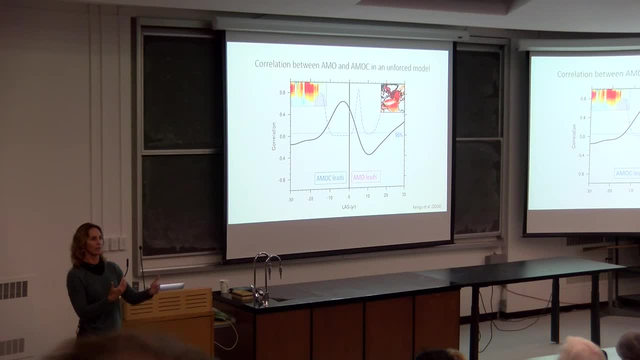 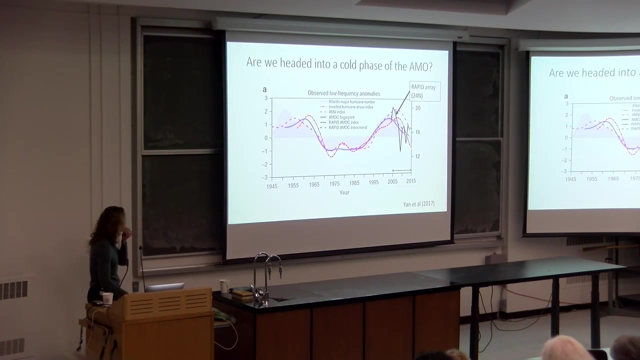 the circulation will appear a couple years later as a warming. Okay Now, so things are just kind of holding together well, And you could take this to a next logical step and say: well, if we have some information about what the AMOC is doing, where are we headed? 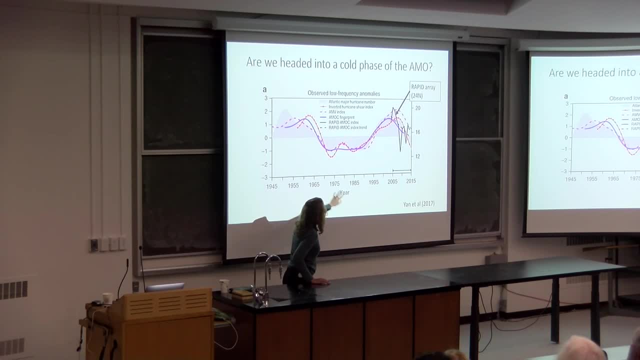 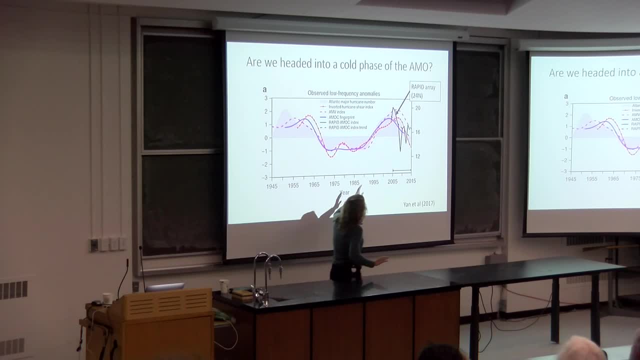 periodicity And if you look at the period of time from 2004 on, you will see an additional black line, which is a collection of observations from an array, an array of ocean observations going from 24 north uh, going across 24 north latitude, from Florida to Africa And uh. 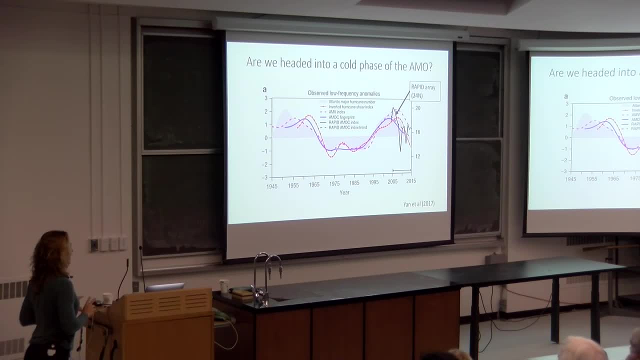 it's a collection of work between my colleagues, um at the Rosenstiel School and and Imt narc in Hawaii and Michigan, Um theulator Michael for its UESP tax at Russian national school Miami, and a bunch of other PIs in the United States and the UK as well, and so 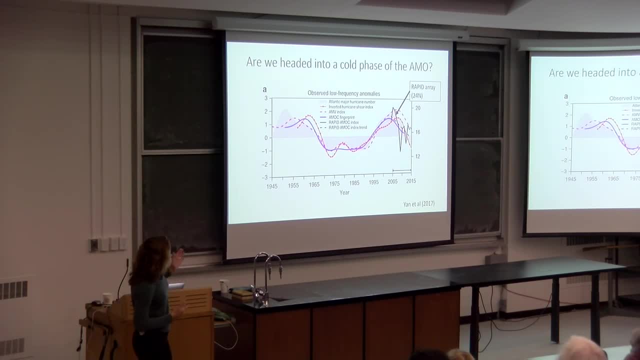 they've been measuring this overturning circulation and we only have, about now, 14 years of data. but you can see, it does seem to suggest that when there's a, when, the when the pink line is going down, it seems to look like there's a, there's a. 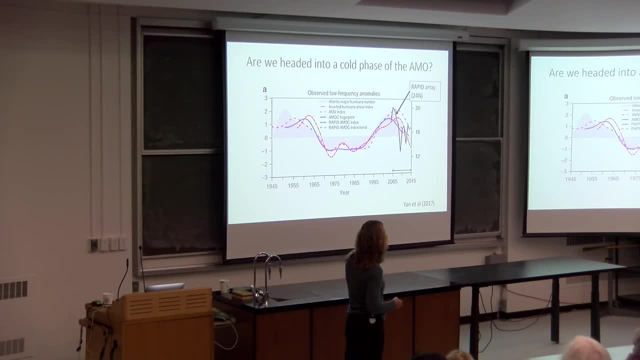 trend in the black, in the black line, which is the observation, so weakening circulation, cooling SST. now you should be getting a little uncomfortable now saying, well, that black line, you're trying to get a trend out of that black line, when you can clearly see that there's a lot of variability. is not so. 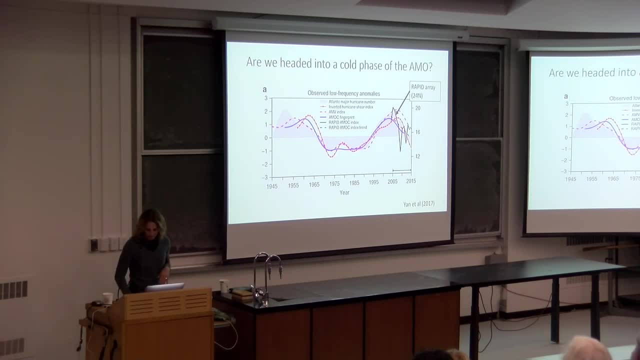 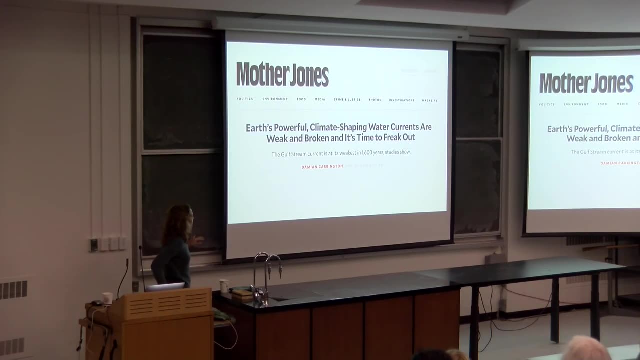 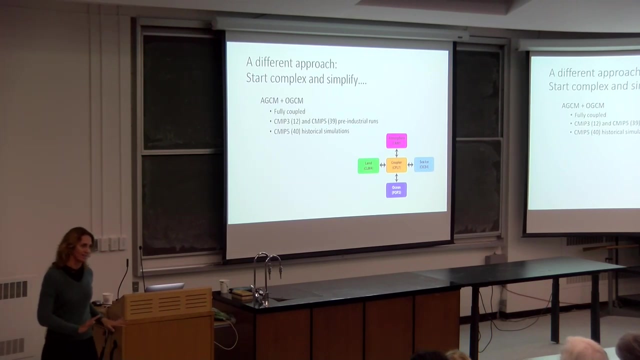 sure about that? okay so, and then, just for fun, I got caught. this is that was a mother Jones article about how this ocean circulation is slowing down and it's time to freak out. all right, so okay, my animations are not not right here, so okay. so, having said all that, now I'm 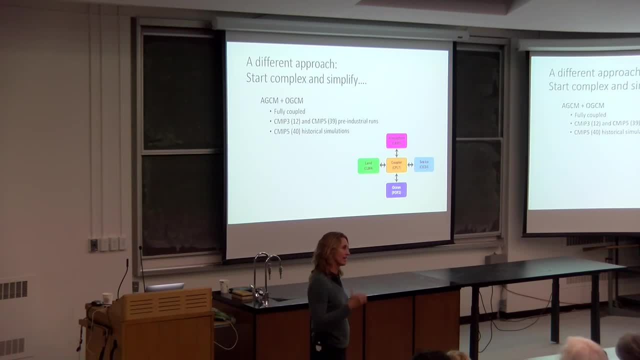 going to make the argument that these ideas have not really been put to a rigorous test. they seem to hold water from lots of different, lots of different lines of evidence. but have we really tried to prove ourselves wrong? and and so that's what I'm- the rest of what I'm going to. 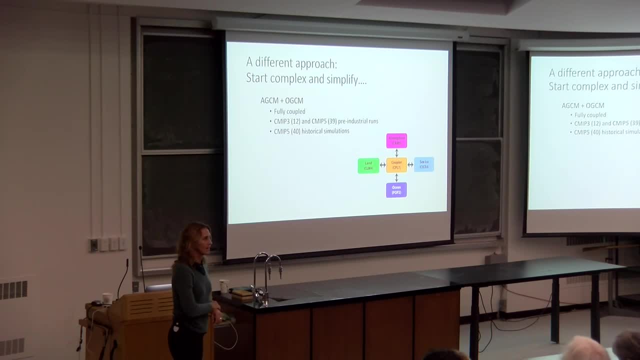 talk about and hopefully I'll make it through. so Paul mentioned that I have been in my work trying to say let's, let's do, let's, let's simplify models, and I'll just tell you right now that what we, what we did with this, which was the innovation in this work, was to take out the ocean circulation. 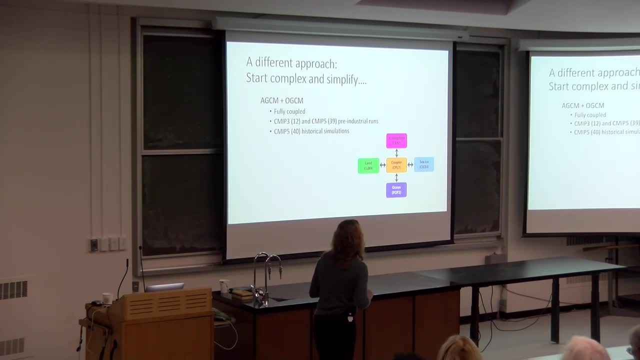 out of a climate model. so let me just give a little bit of background on climate models. I've already mentioned them, but I this is a schematic that I should have written down from a paper by Gen K, so you have an atmosphere which is a collection of primitive equations, or six equations and Navier-Stokes. 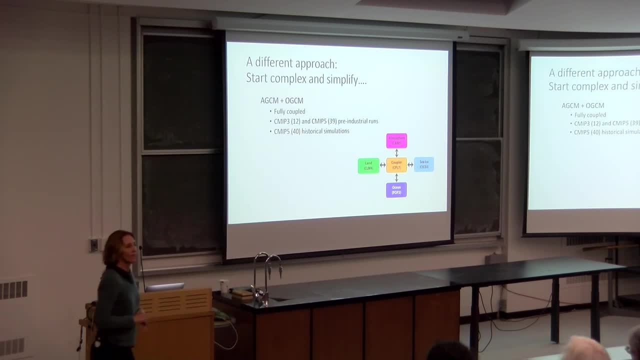 thermodynamics, hydrostatic equation, mass conservation of water vapor, all the you know, familiar things to physicists. it's not rocket science, but it is. it is a computationally very expensive. and then all of the cost comes in the fact that the main drivers of atmospheric circulation, which is the latent heat release is actually happening. 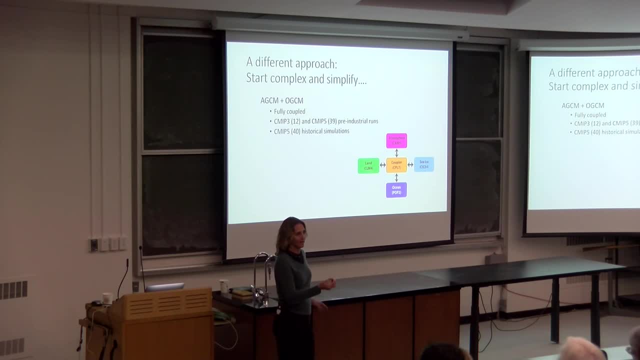 at a scale in the atmosphere that's unresolved by the, by the grid spacing of the climate and or the discretization in climate models, and so there's a whole, whole field of atmospheric modeling where we're trying to represent those sub grid scale processes. okay, so that's the atmosphere. 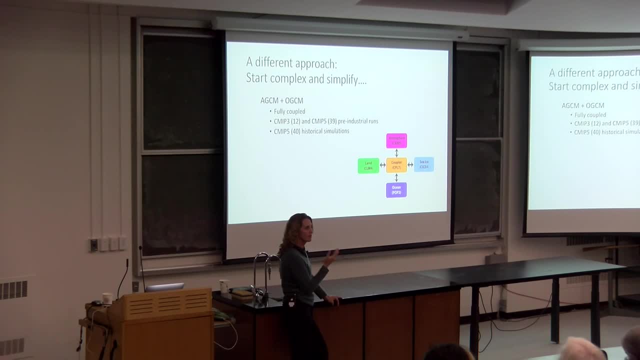 it's coupled to the ocean, exchanges heat, momentum and water. the ocean has a similar set of equations and sea ice model and land models that are that are here as well. this is the standard configuration of this model, which is, in this case, is developed out of the US Center at NCAR. 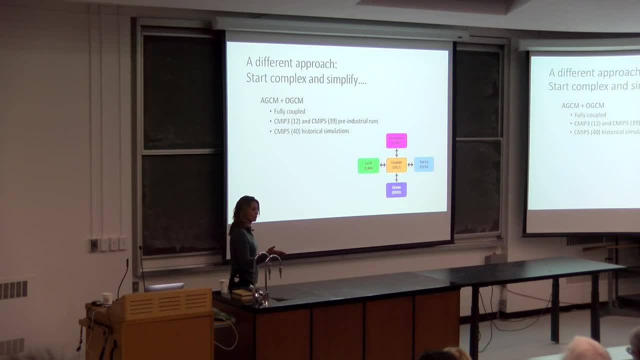 I know that there's a University of Toronto version of this climate model that has been used for lots of different studies, a similar kind of history. So that's my very short spiel on climate models. Then we use them. so I'm going to use them in a few different ways. 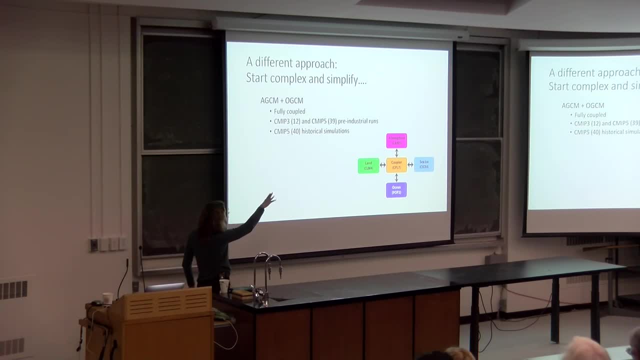 So take a fully coupled climate model where the ocean and the atmosphere can freely exchange heat and momentum and water. I'm going to look at a collection of different climate models from around the world, So they're all part of modeling centers that have participated in a climate model intercomparison project. 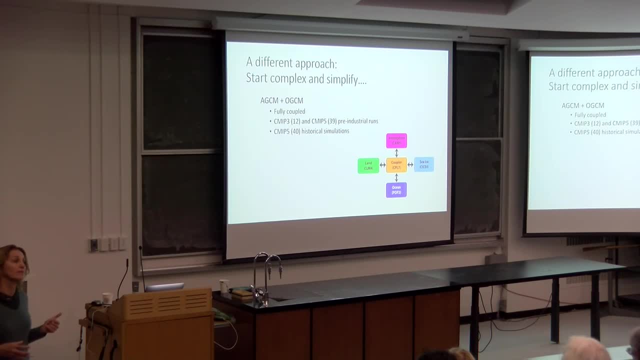 That's what CMIPS stands for. It's really motivated by IPCC scientific assessments, And so there's lots of coordinated experiments that have been in approximately 40 models, And the latest- CMIPS 6,, is going on right now. So all your modeling centers around the world are busily running experiments. 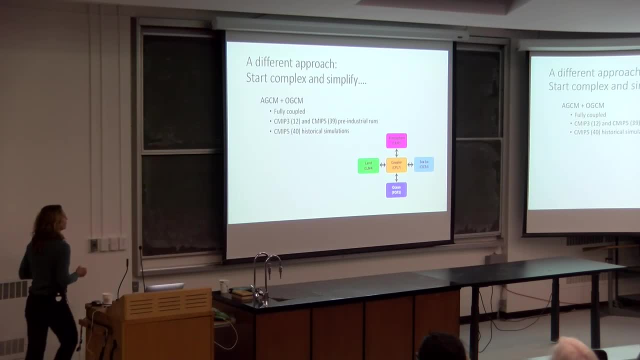 that I'll be able to update you on at some point in the future And then. so now, a really key point is that we have the way we use climate models is I have noted here what we call preindustrial simulations, So this will be ones where we have a stable climate. 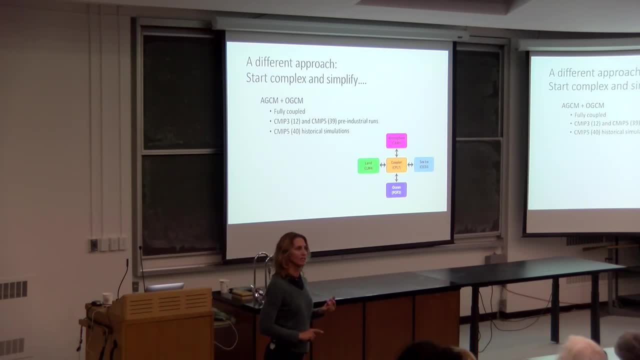 We have stable climate forcing no changes in the sun, no changes in atmosphere, no changes in atmospheric composition, no changes in land surface, no changes in ice. So we're going to look at a number of models here. We're going to look at a number of models here. 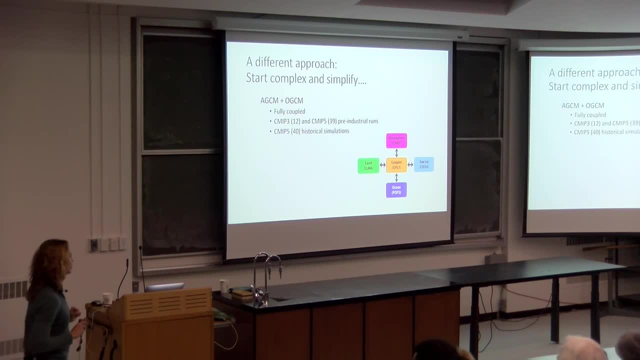 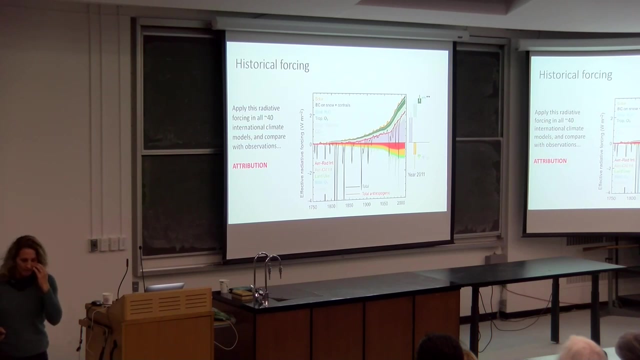 So we're going to look at a number of models here, So you will prescribe these boundary conditions, if you want, and let the model run Now. in contrast to that, our historical simulations- and let me just give you a sense of what that looks like- a collection of scientists from lots of different disciplines have put together 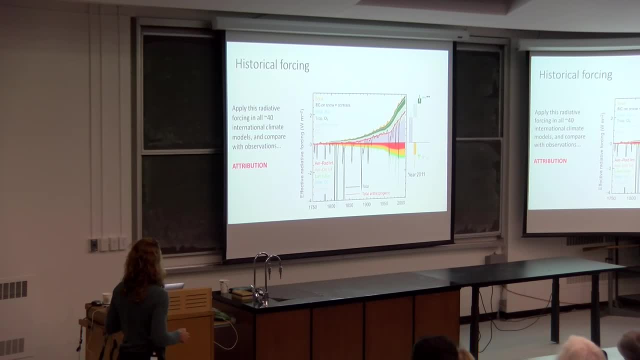 this kind of picture, from the pre-industrial era to 2005 in this case, of all of the different radioforcings. so this is in watts per meter squared of the different here on this side. these are all solar, these are all warming factors for the ocean or, sorry, for the climate. 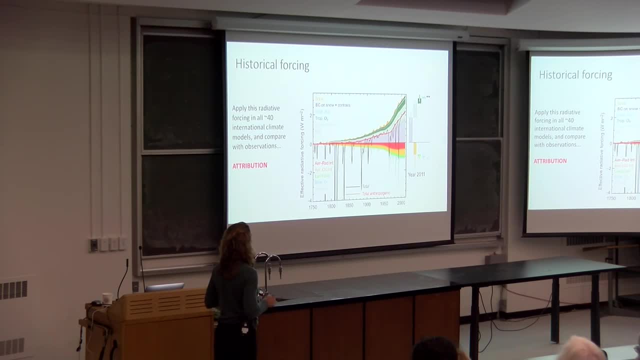 system, the main one being well-mixed greenhouse gases. that's the combination of this gray and these green lines. this gray and green and then on the bottom, here are the effect of aerosols. These are mostly sulfate aerosols that have been increasing over time. but if you notice, 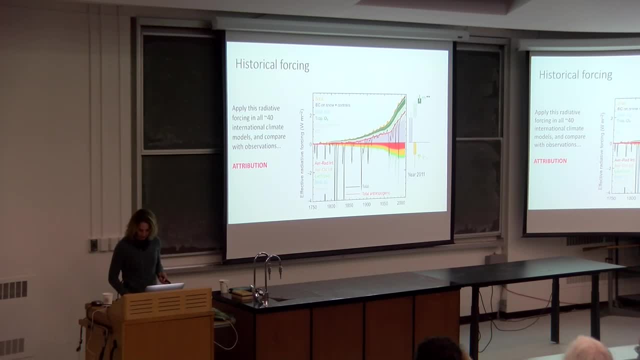 they haven't been increasing steadily over time. oh and just in case you're looking at, you want to know what these are. what are these Paul volcanoes? there's a reason. he's sitting in the front seat here, so okay, so he's a plant. 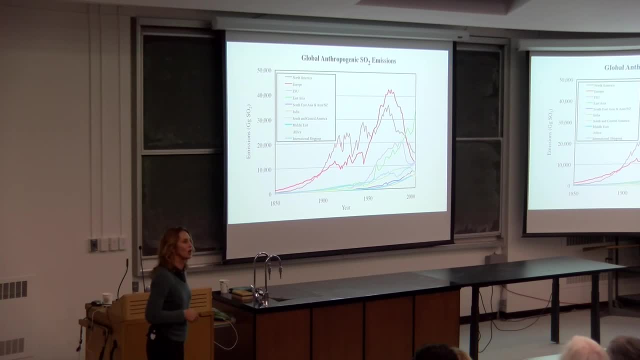 All right. so there's pretty strong multi-decadal variability in the amount of forcing itself, external forcing and what you see here in North America and Europe- so Europe is here in red and North America in pink- are sulfate emissions from these, from coal burning and 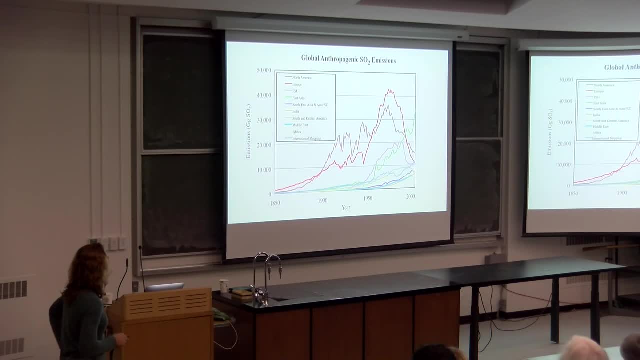 so there's a peak here and there's a decline which coincides with the Clean Air Act of right We're in North America and different and they're European versions as well, and so you have a really a big ramp up, particularly after World War II, and then a big decrease. 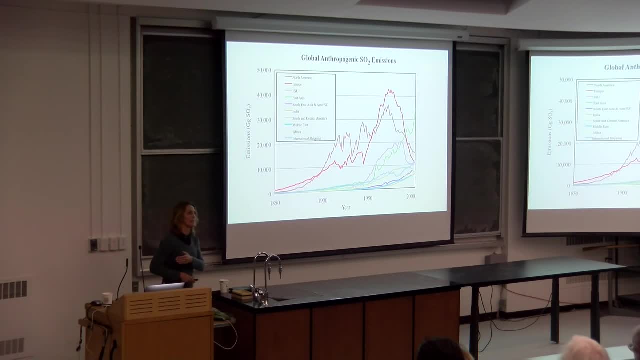 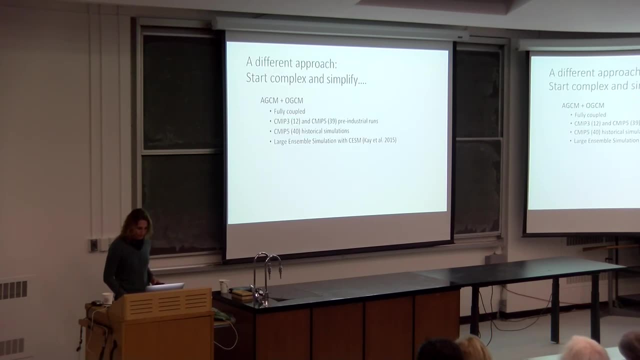 and so what I'm going to show you is that these multi-decadal variations in forcing are a big part of the story of this cycling of the Atlantic Ocean. Okay, so so different approach. So now what we do? What we do is, rather than have an ocean GCM that's moving heat and obeying the equations. 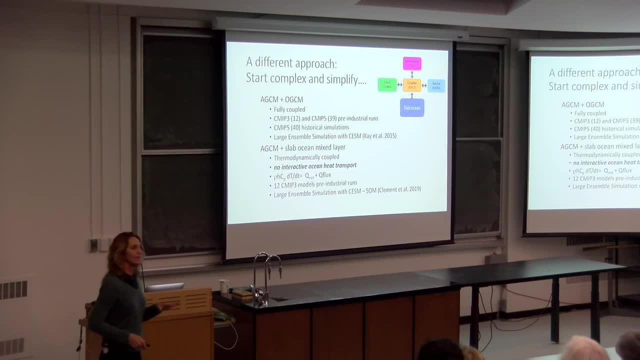 of motion. instead, we're going to replace it with a motionless ocean. that has a really important climate influence of having a large heat capacity. of you know, 50 meters of water is plenty of heat capacity for generating low frequency climate variability. well, I'll. 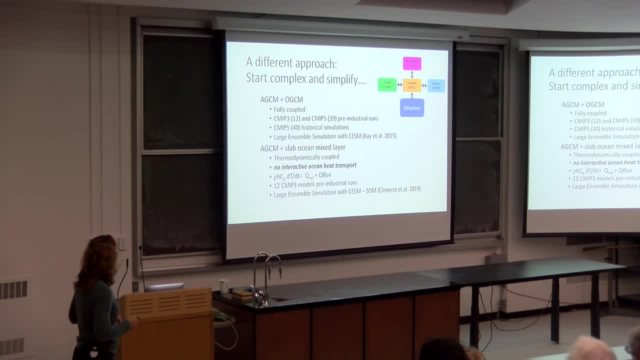 show you that, And so, in this case, the ocean and atmosphere still exchange heat and fresh water, but they don't exchange momentum, And so so we do these, so we'll call these from here on atmospheric GCM slab-ocean mixed. 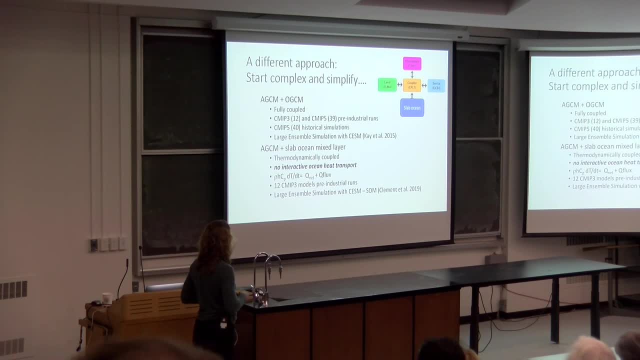 layers. The same kind of experiments have been done with lots of different climate models so we could be able to compare across models. and then we've done a number of these simulations with a NCARS version, with a slab-ocean, with NCARS model, with a slab-ocean model. 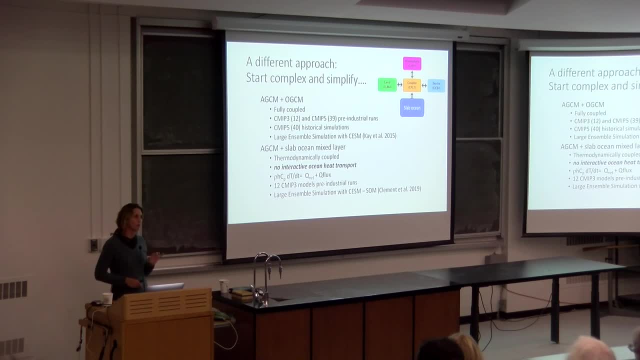 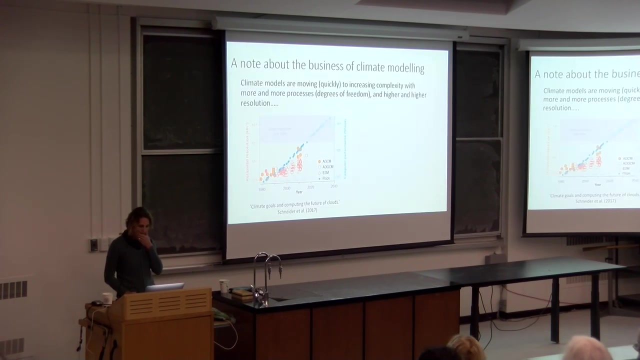 Okay, so really simple here, All we're doing is taking the exact same model configuration, all the same physics, but swapping out an ocean that moves with an ocean that doesn't move. I'm going to run out of time, So what I was going to go on is I was going to go on a little bit longer, but I'm going. 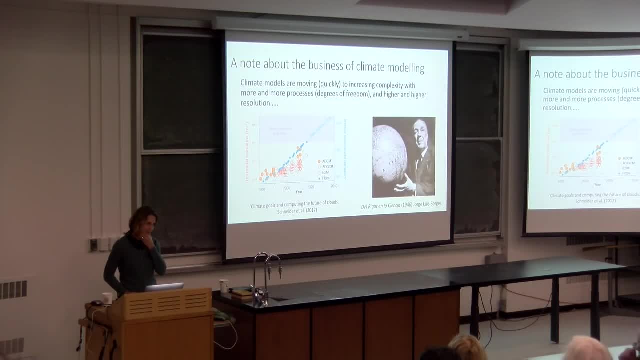 to go on a little bit longer, Okay, Okay. So I'm going to go on a slight tangent about how doing this kind of simplification of the ocean, of the climate system runs real counter to the way that our field is evolving with. 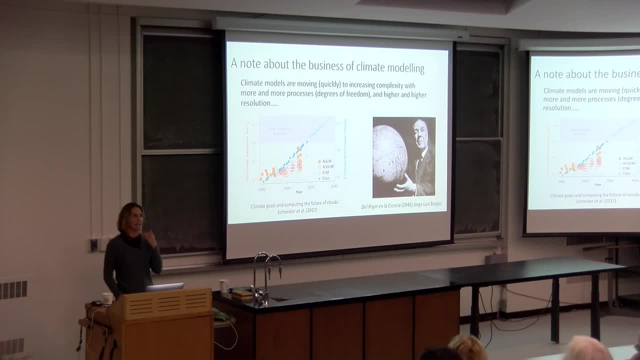 quickly, quickly increasing complexity and higher and higher resolution. Okay, I will permit myself this one nod to Jorge Luis Borges, who's an Argentine writer, who wrote about a country that made commissioned a map of their country, and they got so detailed. 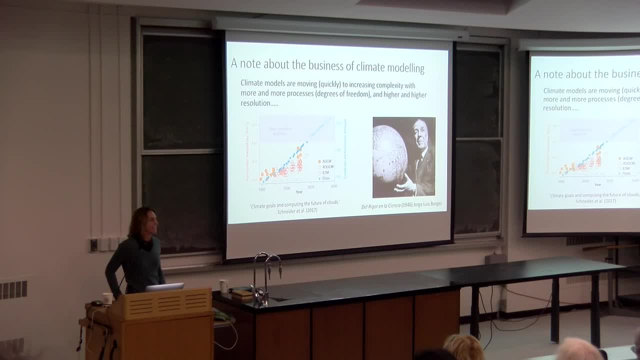 that the map of the country was the same- The size of the country- And then the story ends. the short story ends with the map being torn up in tatters and rolling through the countryside. It was of no use to anyone, So anyway, cautionary tale. 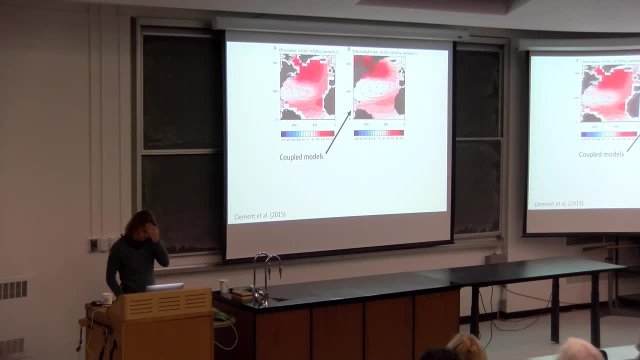 I can come back to this if people are interested in the sort of trends in climate modeling, but I'll just want to jump quickly to the results. So this was the picture that I showed way 45 minutes ago now of the, you know, of the. 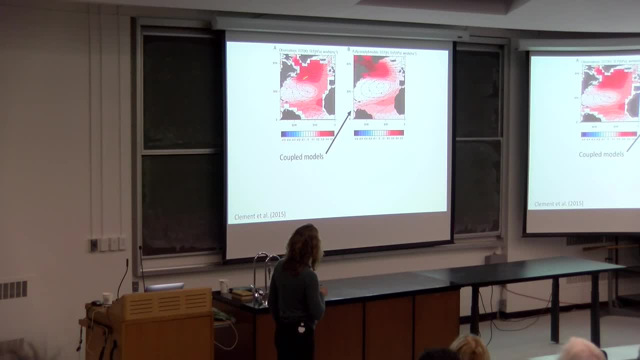 Atlantic surface temperature, warming and cooling, with winds and sea level pressure on top. If you do the same exact calculation in the climate model, you get something that looks a lot like the real world, not only in terms of surface temperature, but also in terms 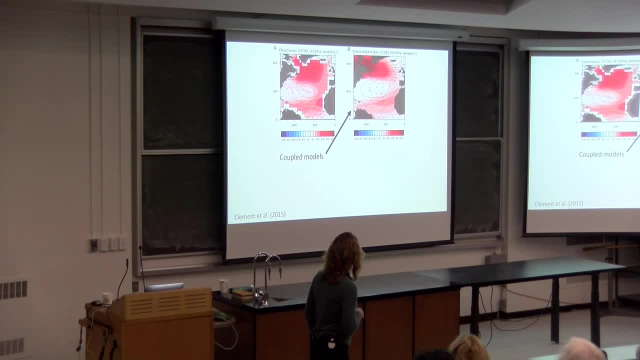 of the winds that go along with it and the atmospheric circulation that goes with it. Now, if you were, if you were interested in saying: okay, I'm pretty sure that it's the AMOC that does this, and you take this index and correlate it with the AMOC, you will get. 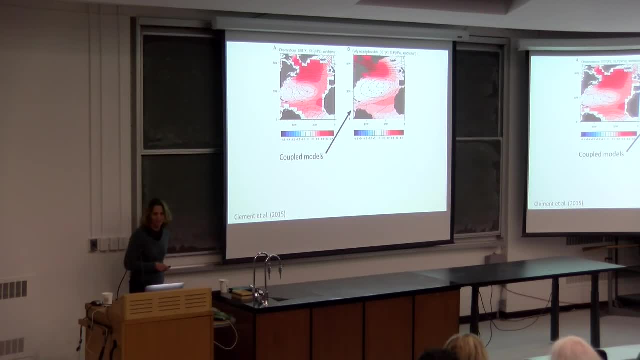 a positive correlation, right? Paul? and his former student or former postdoc, Neil Tandon, did that and you do see there is a correlation between them. Okay, so I think I've you know you could convince yourself that you have explained. 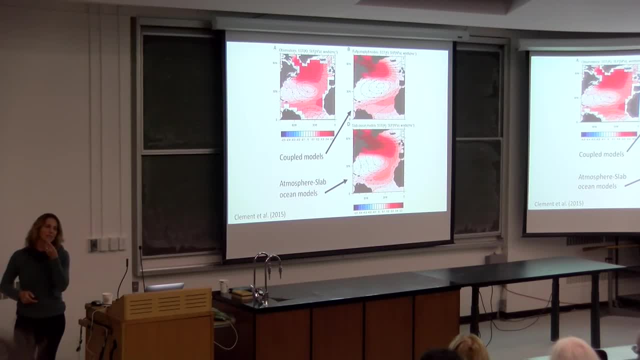 the observed world, but then we do this in the models that have no interactive ocean circulation and there's really no difference between these two. If anything, I would say this has some looks slightly more like observations in some ways than this does. 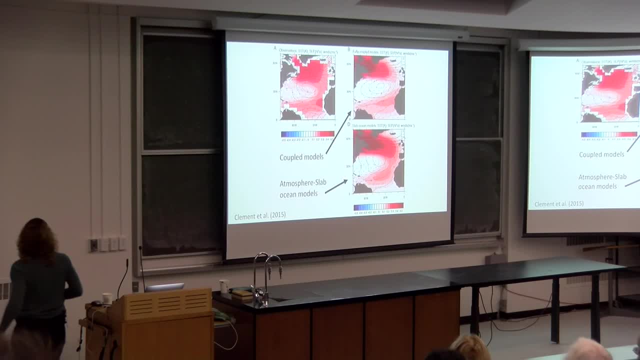 And so you can have, you can generate this variability without an ocean, without varying ocean circulation. So now you should be saying: well, hold on, we. I started out the talk saying the ocean was important because it introduced a long time scale, so maybe the pattern is the same. 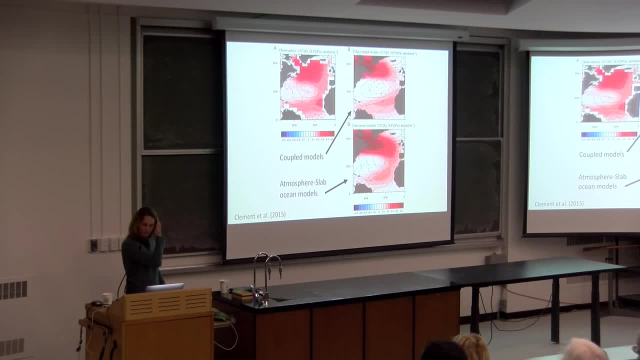 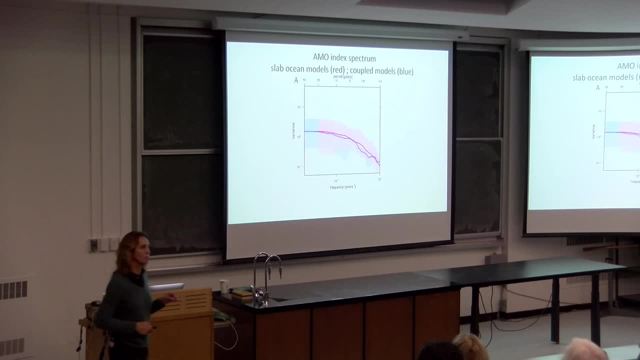 but the time characteristics are different, And so you would think that the pattern of this mode of variability are different, and this is an answer to that. If we take the a power spectrum of the index, so we look at periods from 1 to 50 years. 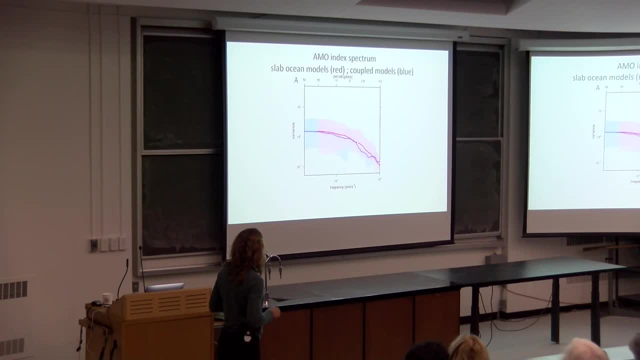 and shown on here. the red, the red line and the pink shading around it is all estimates of the power spectrum from all of the slab ocean models And the blue line is the coupled models. So we argue you cannot distinguish between these two power spectra. 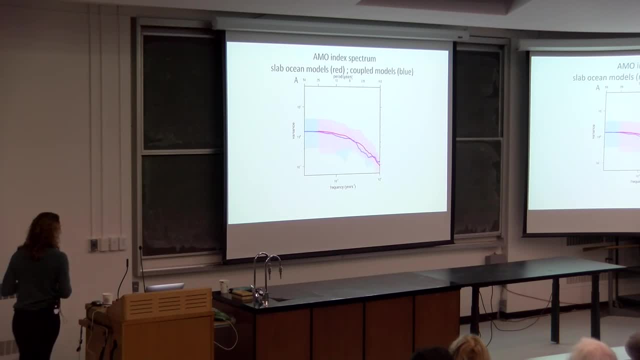 The time and space characteristics of this phenomena don't seem to be altered by the presence of a variable ocean, And so the purpose of that paper says these words: interactive ocean is not necessary to produce AMO in these climate models, And the climate models look like observations. so we can make the next step. 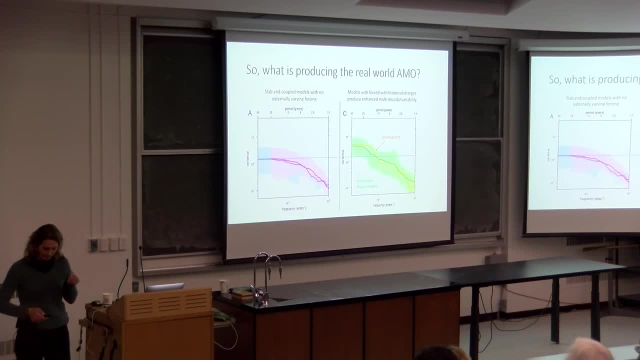 Now here's where the story is not quite so clear. If you take this power spectrum and compare it now with observations- the observations are shown in orange here- you see that there is a lot more power at multi-decadal time scales in observations, to the extent that we can believe a power spectrum. 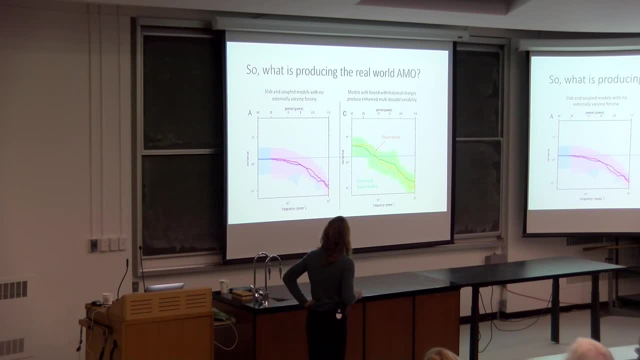 based on just two realizations here of this time scale, But there is more power. And then if you look at models that include these multi-decadal fluctuations in atmospheric composition and in particular sulfate aerosols, you see that there's a lot more variability. 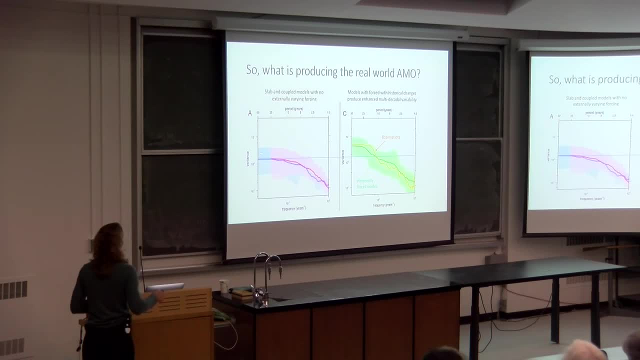 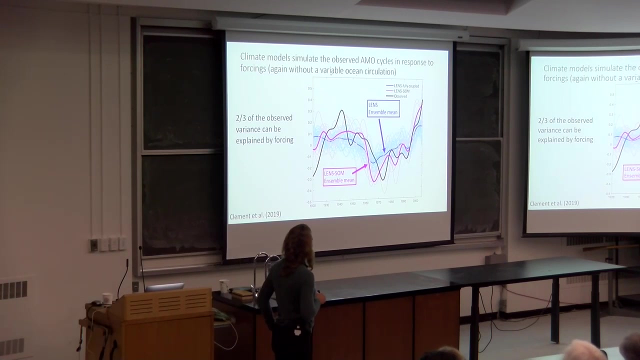 in observations and models than there are in these models for the pre-industrial, where the external forcing is not, And then this is almost over. but just to prove to you that there is, if you take a climate model and you look at the compare, a climate model simulation of the AMO in its 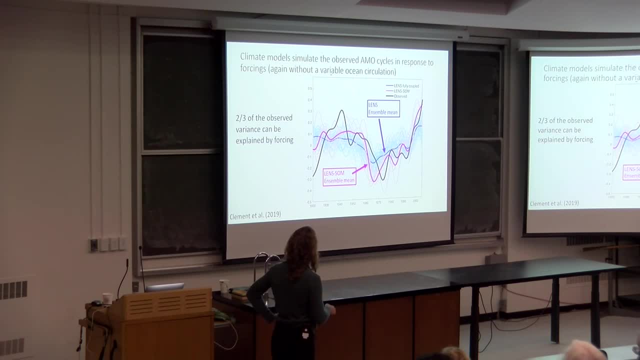 time history with the observed. so the observed in this is black. here's 1920, 2005,. here's the black which is showing the observed AMO, And then you see that there's a lot more variability. So the blue line in here is the average of 40 different simulations with the climate. 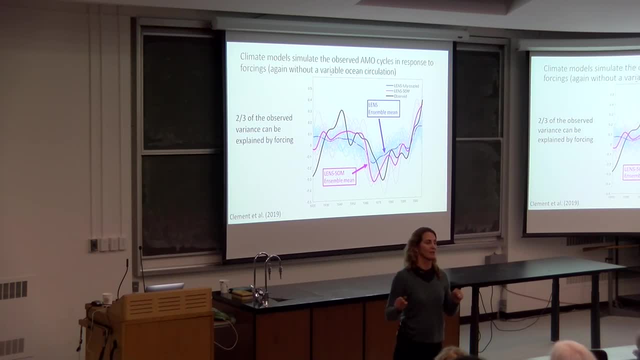 model, all with the same external forcing but slightly different initial conditions. So each bit of this wiggly is different in these 42, but the average of them. the only thing they have in common is the time varying forcing. So this, the blue line, is an estimate of the forced response. 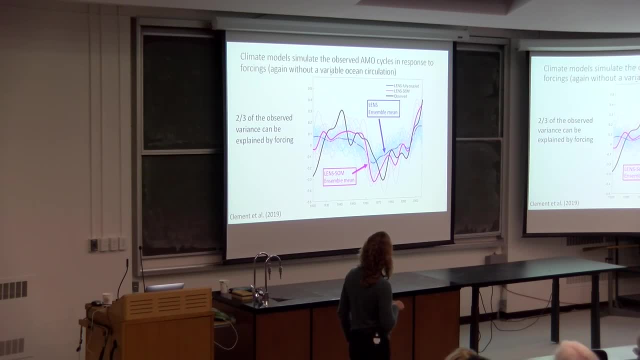 We did the same experiment using replacing the blue line, So the blue line is an estimate of the forced response. We did the same experiment using replacing the blue line And then we did the same experiment using the ocean, with a slab ocean, and that's shown. 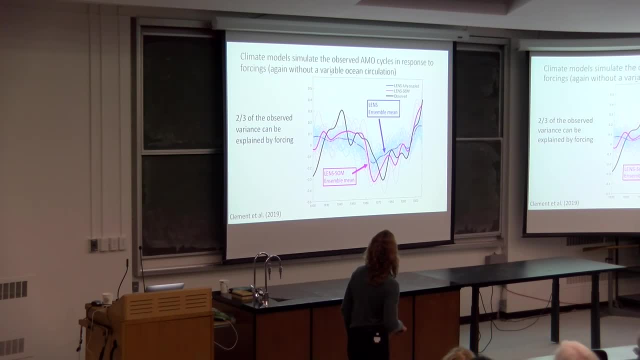 here in pink, And I think what you see is there's a good relationship between, in fact, 2 thirds of the explained variance, the correlation coefficients of about .8.. So about 2 thirds of the explained of the variance of this line can be explained as: 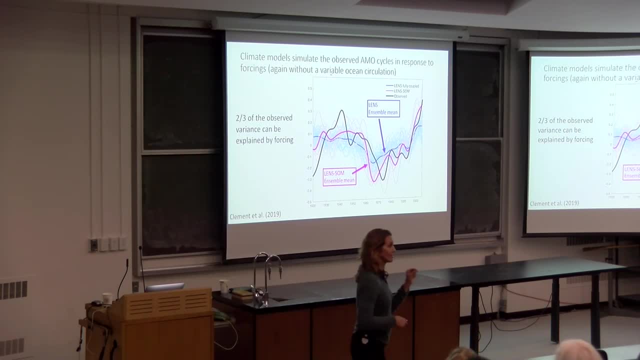 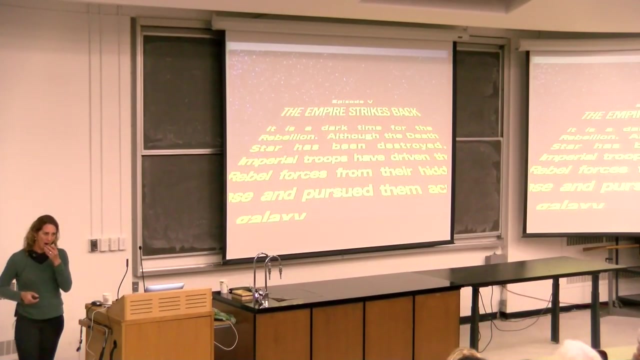 the response to climate forcing. and not just climate forcing but just the ocean thermal response to force climate forcing, so without any changes in ocean circulation. okay, so we've put. we've written lots of papers on this topic. it was not a very popular point of 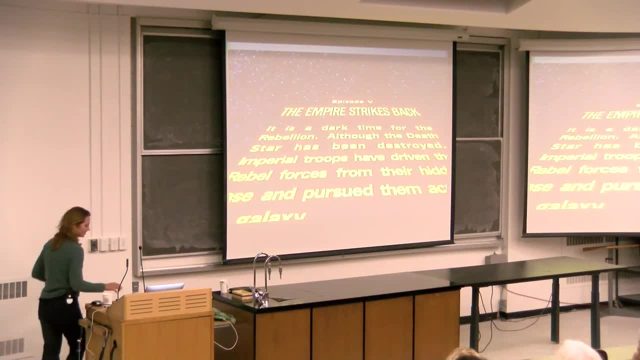 view, and I will just so. there were a bunch of different papers that have been published- this is actually just a just a few of them that have been published- saying, well, this idea can't be right, and so I should say I'm making kind of a joke about it, but it is. it has been, I think, one of the most exciting times in. 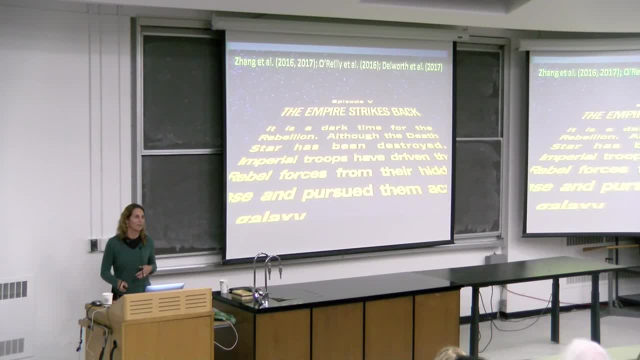 my scientific career to be really at the at the center of what is a really like hot-button debate about which I think has really big implications. I had 15 years of experience in the scientific field, and I had 15 years of experience in the scientific field and I had 15 more slides on how this debate has pulled has. 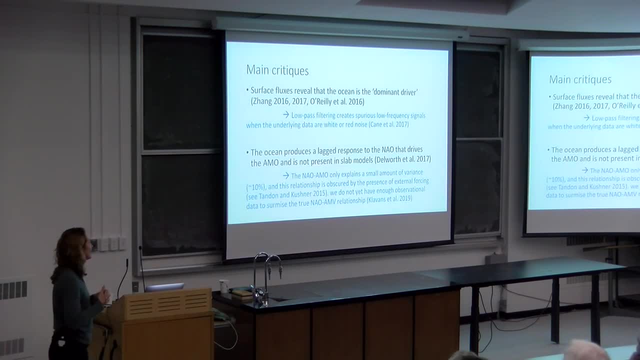 more slides on how this debate has pulled has more slides on how this debate has pulled has has played out and since 2015 has played out, and since 2015 has played out and since 2015, and I will, just I am NOT gonna go through. 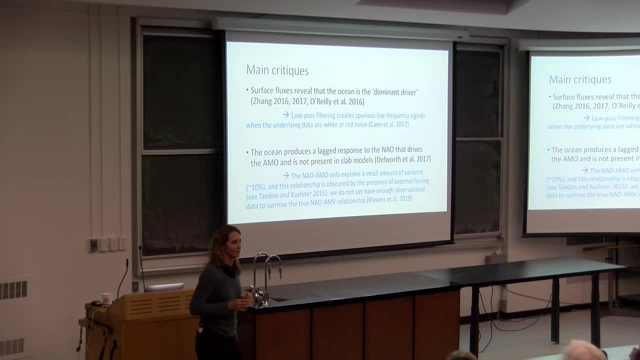 and I will just, I am NOT gonna go through and I will just I am NOT gonna go through the details of that back and forth. now I the details of that back and forth now. I the details of that back and forth now, I think, because I think what's that I have? 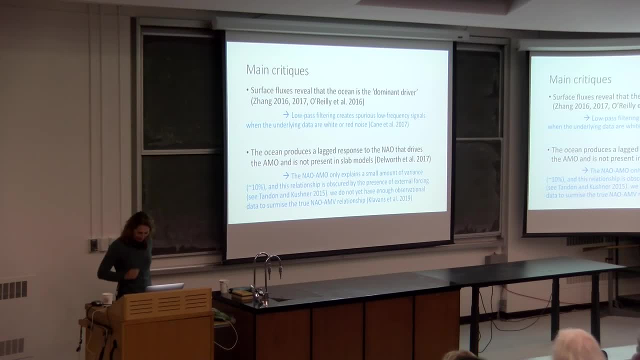 think because I think what's that I have? think because I think what's that I have 10 minutes, okay, all right, 10 minutes, okay, all right, 10 minutes, okay, all right. so, So does that mean you want to hear the story or not? Yes, OK, I'm getting the thumbs up. 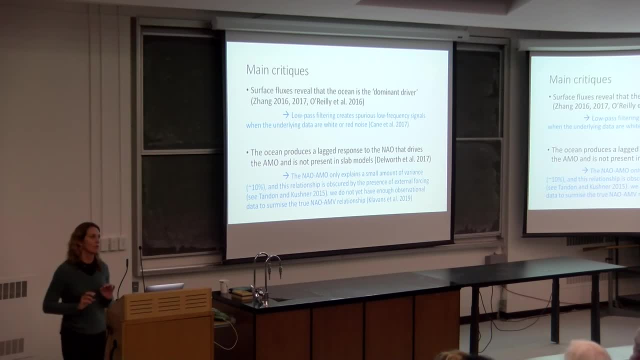 All right, so I'll just say in words what it was. So a bunch of papers showed that you were trying to argue that you could use the surface heat fluxes in order to infer what was driving what. So if you had the atmosphere driving surface temperature, anomalies. there would be a heating of the ocean, a heat transfer from the atmosphere to the ocean, And so that would have a particular sign of surface heat flux would be into the ocean. On the other hand, if you had the ocean driving the surface, temperature anomalies, that you would actually be converging heat, which would result in an increase in temperature, And that alone would produce a heat loss from the ocean, And so the prediction is that the atmosphere is driving. you have heat going into the ocean when it's warm. 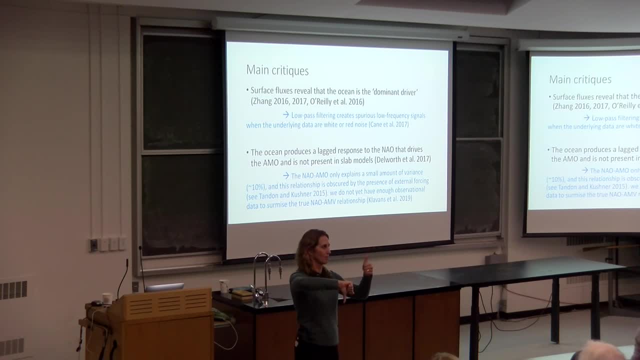 And if the ocean is driving, you have heat going out of the ocean when it was warm. OK, so that makes sense. I see a head nodding in the back, But the complexity of this is that all of this data is low-pass filtered. 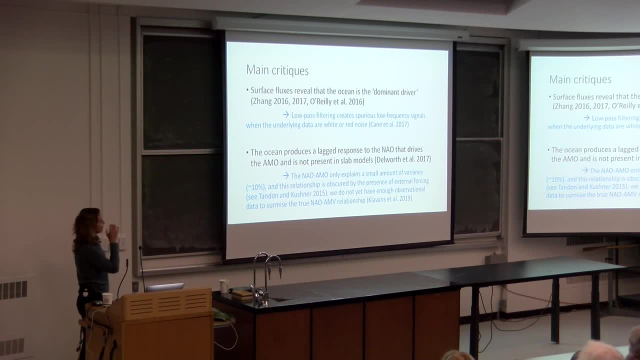 And so this paper, which I'm happy to share with you, was arguing that this low-pass filtering is actually creating signals Which are in the surface fluxes, which are easy to misinterpret. That's probably not a very satisfying answer, So that kind of is in the weeds about how. 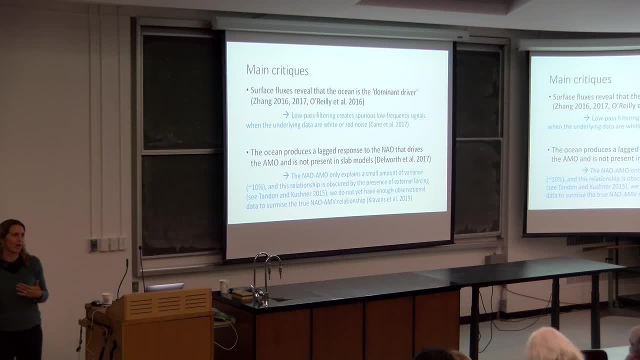 do you diagnose what's driving what in a system where there's a lot of correlated variability? So let me leave that one aside. I think the more accessible debate was the fact that the real world ocean seems to have a lagged response To the atmospheric circulation. 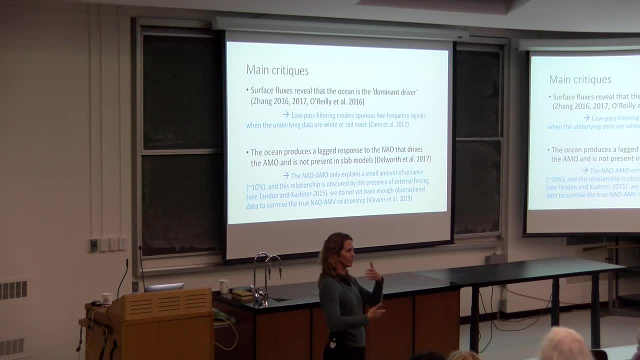 So, while I showed you the picture of the simultaneous correlation between the ocean and the atmosphere, there's a lagged response that is not present in the slab model. So the real world and coupled models seem to be doing something that's slightly different And, in other words, it's a lag. 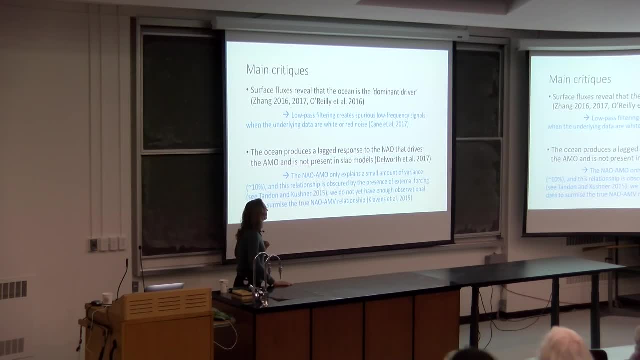 In other words, the ocean is doing something, And our reply to that, which is in a paper by a student who, Jeremy, just in review right now, that the relationship between the atmospheric circulation, the NAO and the AMO only explains a small amount of the variance. 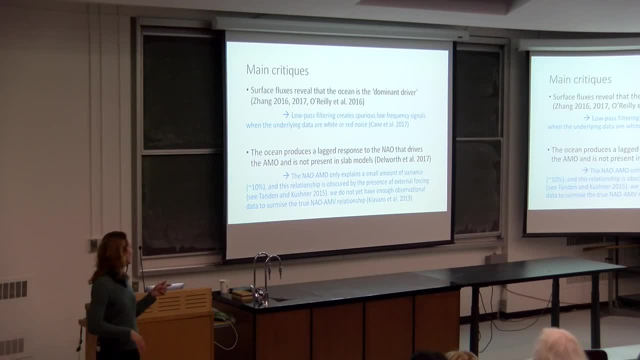 But more importantly- and this gets back to work that Paul has done, where, if the main driver, I already told you two thirds of the variability could be explained by external forcing. So the main driver of sea surface temperature variability is the external forcing. 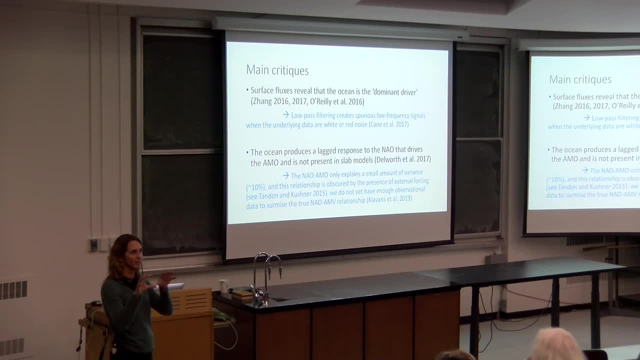 And you're looking for correlations between noisy fields in the atmosphere and the ocean that you can actually get really. you can obscure those relationships when the main driver is something else, And then we conclude by saying we don't have enough data to understand the true relationship between. 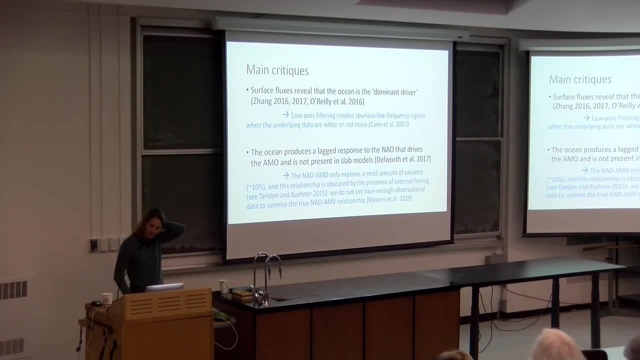 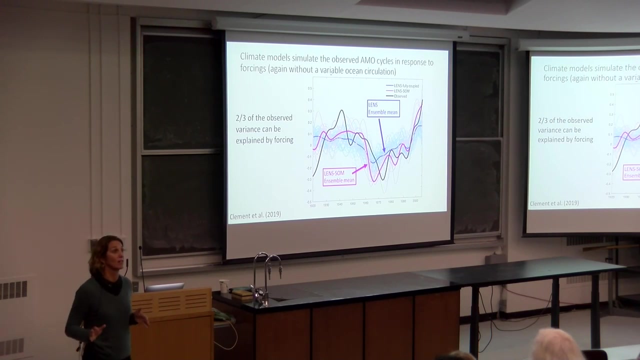 The ocean and the, or to the NAO and the AMO. Okay, I shouldn't. I'm sorry, I shouldn't have taken that. I I. without going into the details, I'll just we. there's a back and forth and an ongoing debate on both of the. 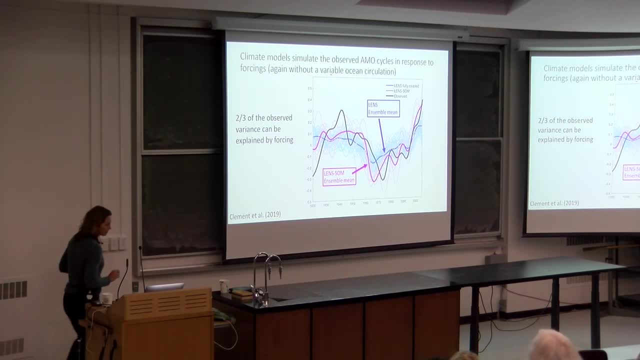 in both of those areas. So back to this, and I'm going to try to wrap up real quickly now. So back to this result: that two thirds of the observed variance can be explained by forcing, If that's the case, but it still leaves a third. 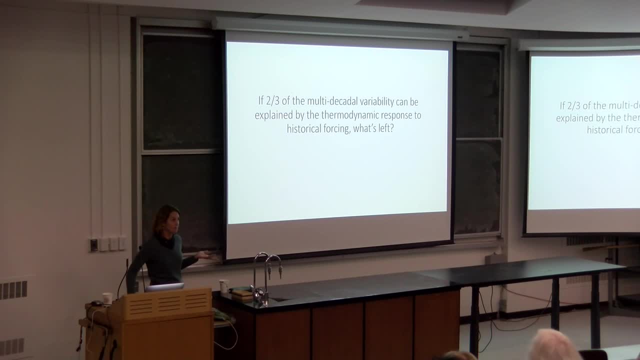 of the variability on which is might be something that you'd be interested in. I mean, as a, you know, as a climate scientist. I don't know what a physicist's perspective is, but if you've explained two thirds of the problem, you've done a pretty good job. 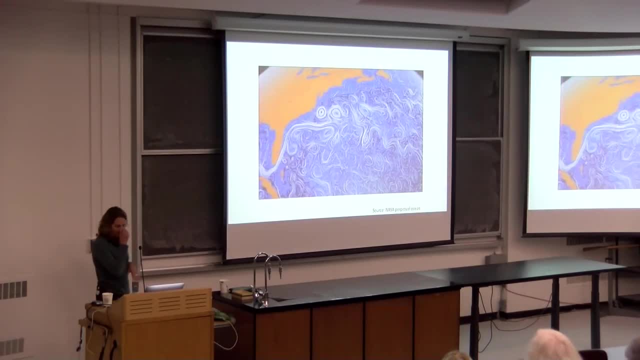 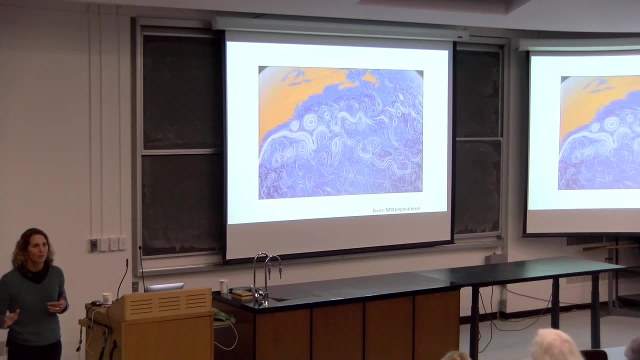 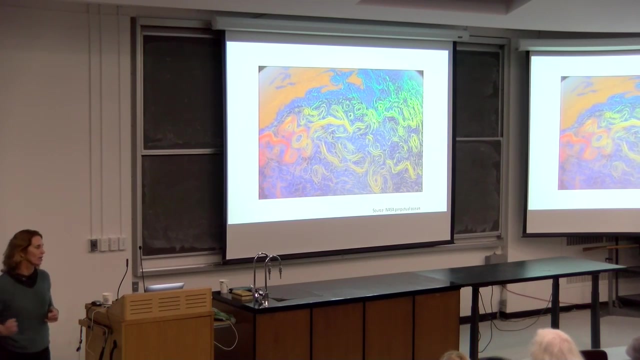 We'll quit there. but so so I I'm going to say, since the period of time when these ideas about the AMOC were evolving, the early climate models and early ocean observations, we've learned a lot about the real world ocean. 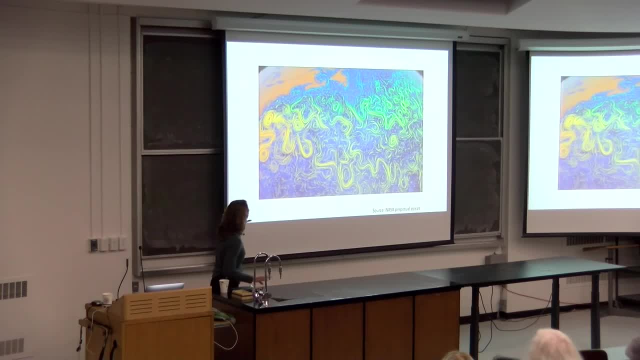 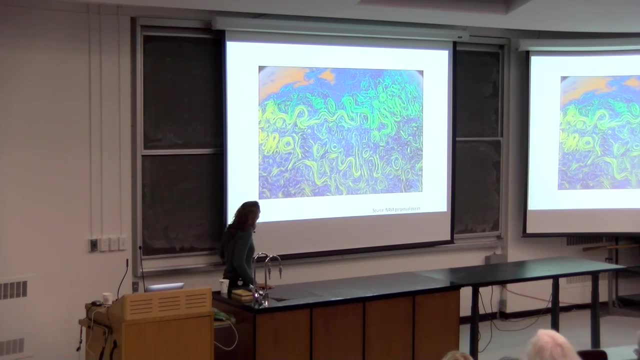 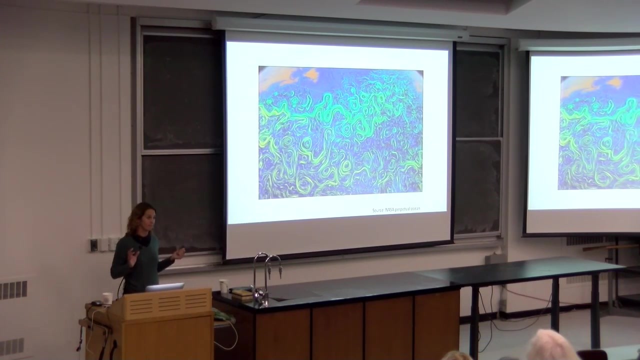 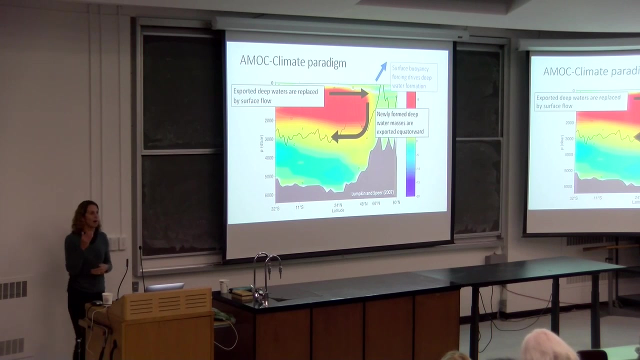 And in particular, this is a movie from an ocean, high resolution ocean model. You may have seen this if you've been in Nicholas's classes, that the real world ocean is really noisy, Okay, And so this picture of the AMOC being the dominant mechanism. 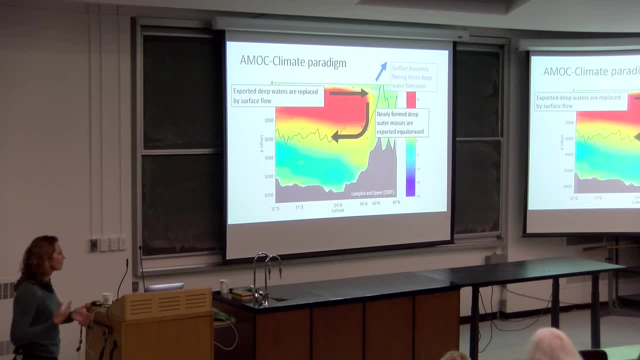 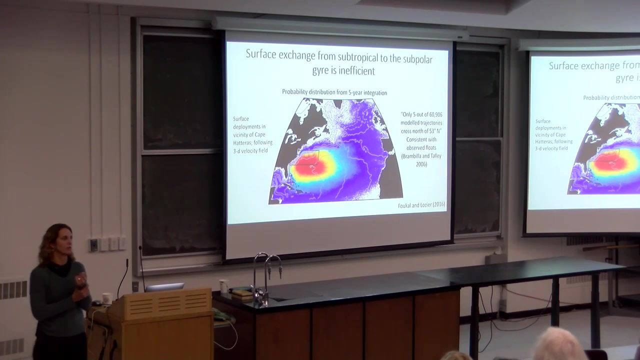 of importance for climate in the ocean is probably an oversimplified way of looking at the ocean circulation, And I'll just give you a couple of examples from work that I've been very influenced by: by Susan Lozier, who's an oceanographer at Duke. 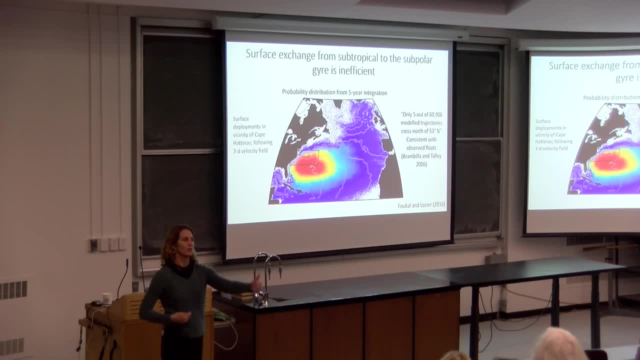 Looking at this idea of a coherent overturning circulation in the ocean. This is a picture of of a tracer experiment, where they deploy tracers in that box and watch how they get advected around in a high resolution ocean model, And so the colors show the density at some five years. 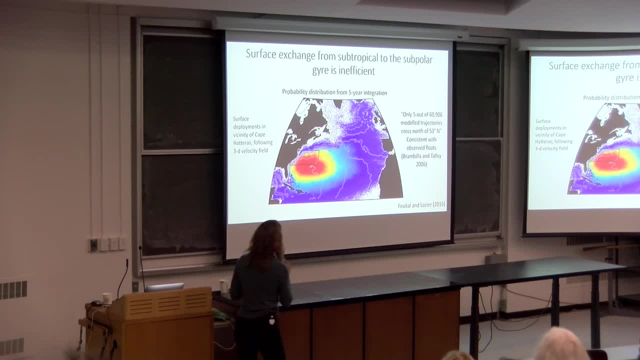 after the deployment, So in a five year time frame, almost all of this waters that would in the sort of the AMOC paradigm, which would be happily going up to the high northern latitudes where they're going to sink- almost all of them stay. 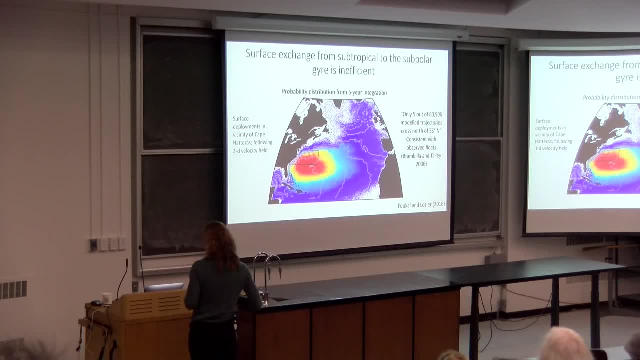 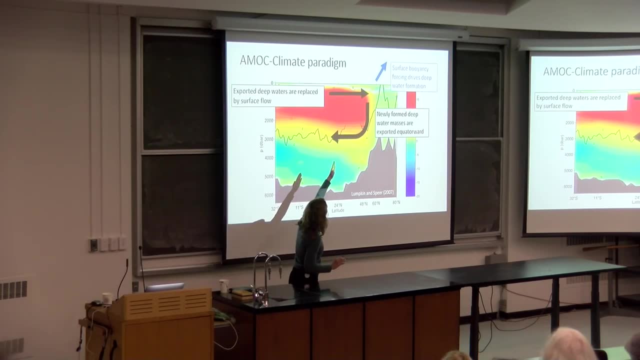 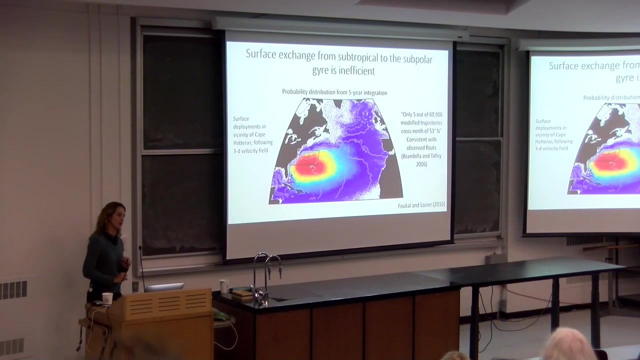 within the subtropical gyre. So there's this, this idea of that you have an efficient exchange of surface waters between the subtropics and the extratropics. It's not borne out by modern day oceanographic tools. So this is a. this is a. this is from a model simulation. 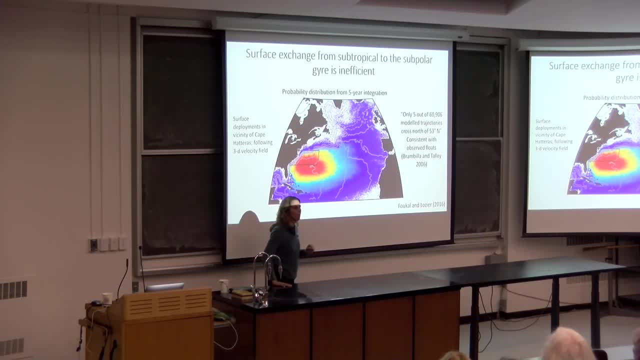 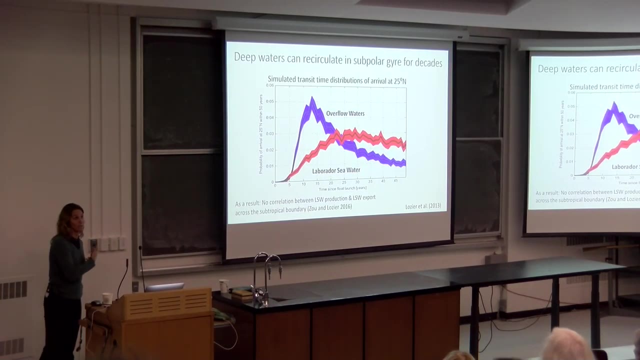 but they also cite that, with observable floats that are put in the ocean, that there's a very inefficient exchange between the tropics, or the subtropics, and the extratropics And similarly the in the deep waters. so this deep returning part, we think of it as this sort. 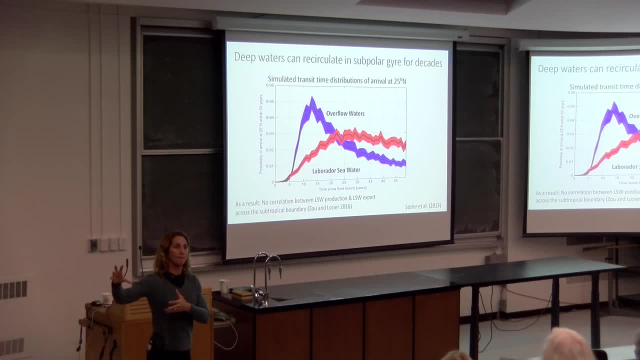 of efficient exchange of deep waters from the subpolar basin out, which is an important part of heat, warm water in cold water, out net heat transport to the north, And one of the things we see is that it takes these waters of decade or longer to actually get exported from the gyre. 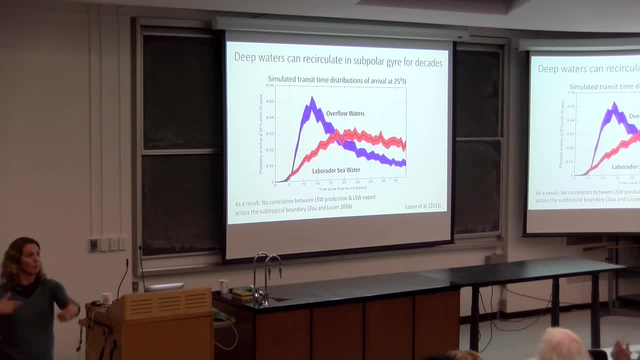 So this idea that we can have, you know, have this overturning circulation that would be coherent on these timescales of decades, even multi-decades, is not really supported by modern oceanographic tools which are telling us that the ocean is really messy. 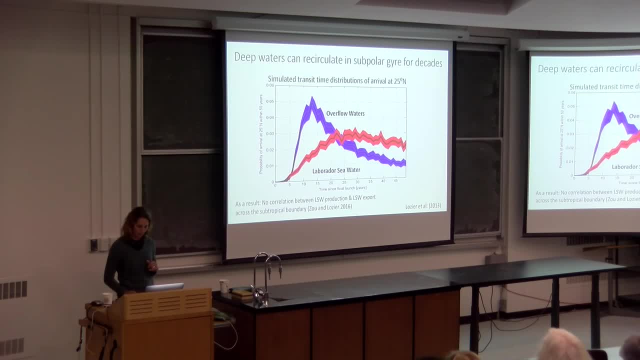 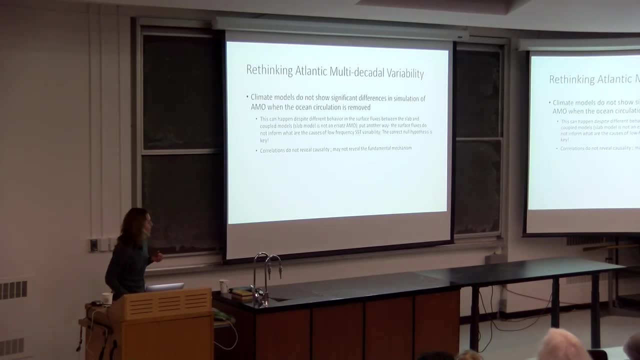 And this paradigm for thinking about the ocean circulation and its role in the climate, I think is oversimplified. So just to wrap up, some concluding remarks. So climate models: Climate models do not show significant differences in the simulation of the AMO. 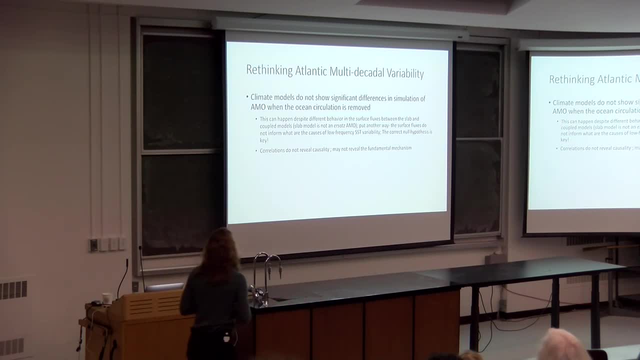 when the ocean circulation was removed. So that was our main finding And this can happen. So this is the debate- can happen despite changes in the surface fluxes. In other words, and just as some final points, that correlations in this case do not reveal causality. 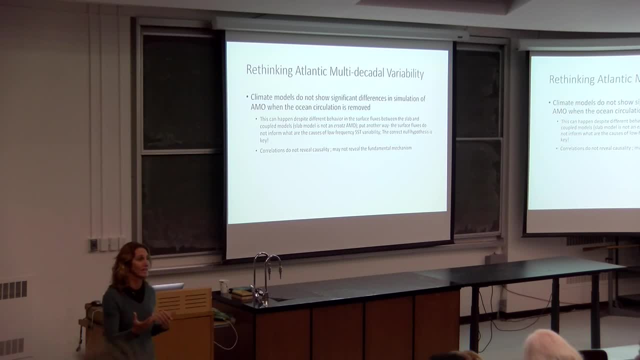 and cannot reveal the fundamental mechanism, And so we needed to come in and do this intervention in the model in order to understand, really as a test, of one way of testing, whether the ocean circulation is important. The external forcing plays a role in explaining these cycles.